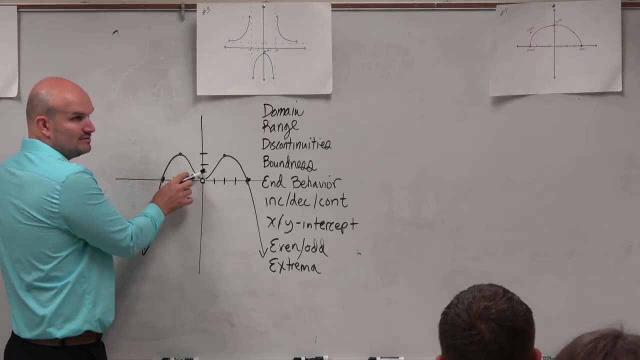 Because even though there's undefined value here, there's a point above it. So it's covered, right, So we're covered in that respect, And then it just continues. It continues going to the left and continues going to the right. So I saw a couple of different pieces of notation. 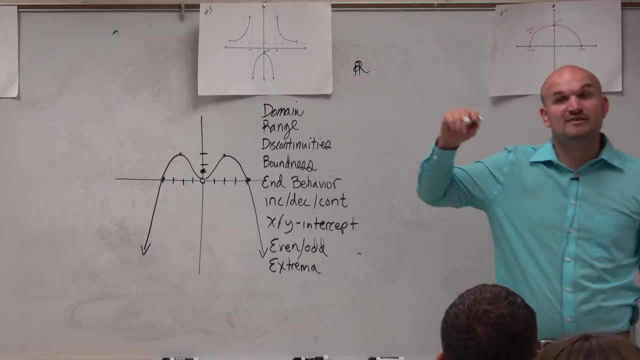 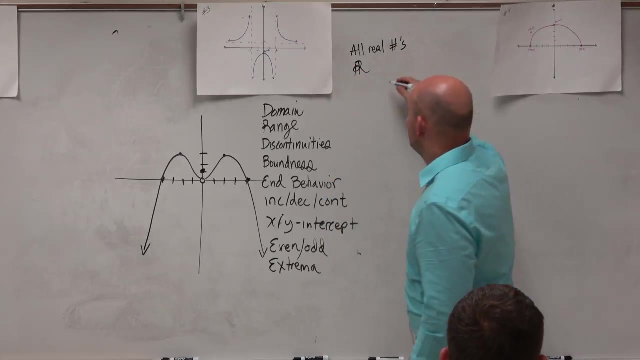 from previous classes. They said: all real numbers like this. Some even wrote out all real numbers. They wrote like that. Some people even wrote this. They used inequality notation, which is perfectly fine. Those are all OK. And on a free response, depending on what my directions are. 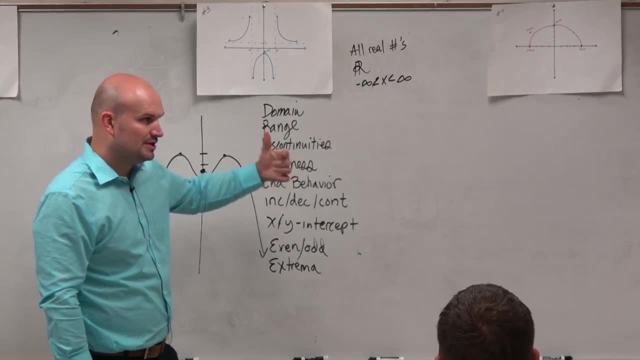 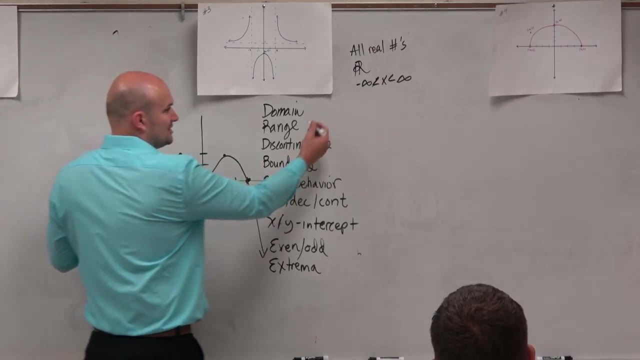 those would all be acceptable. In this class, though, we're primarily going to be working with interval notation, And interval notation is basically saying how far left to how far right, So you're basically just creating an interval of one value to the next. 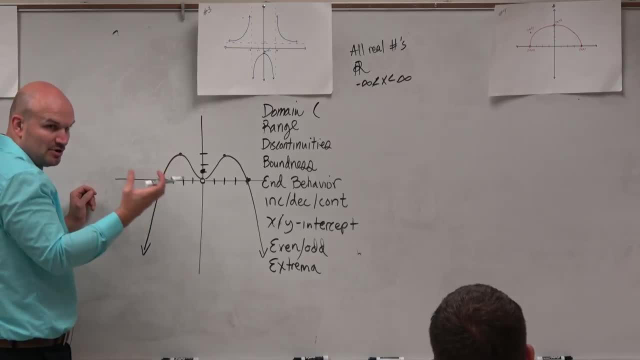 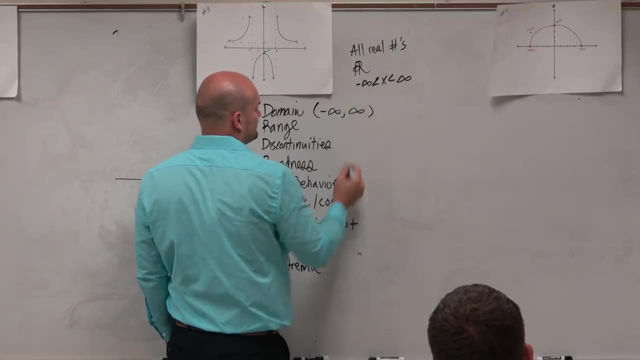 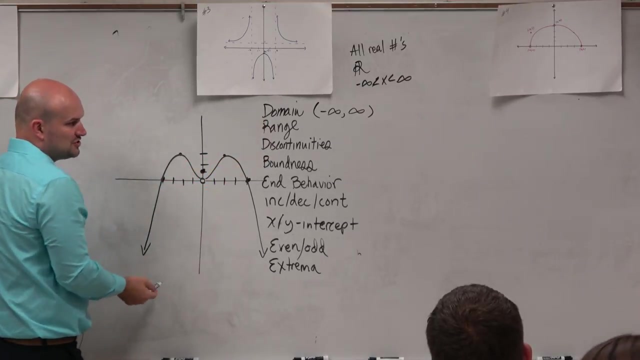 And since infinity is not actually a number, you can't have infinity of anything it's not contained. So that's why we use a parentheses rather than a bracket. On contrary, the range. if the domain is the set of all x values, the range. 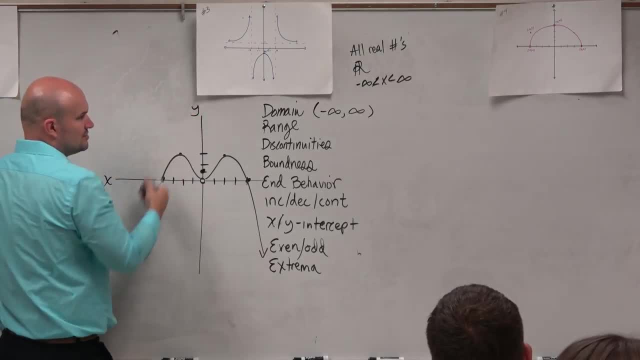 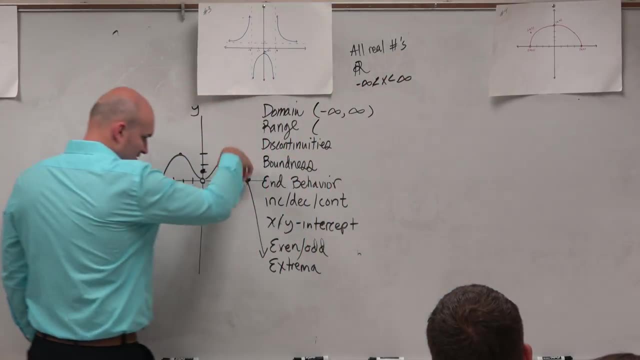 is the set of all y values. Here's x and here's your y. So the range is the set of all y values, basically asking us how low does the graph go to? how high does it go? So the lowest the graph goes, it looks like it's continuing all. 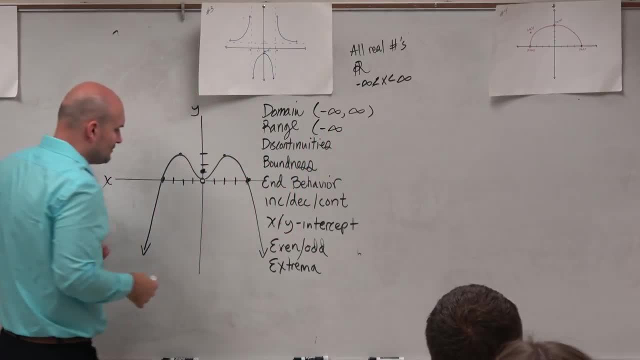 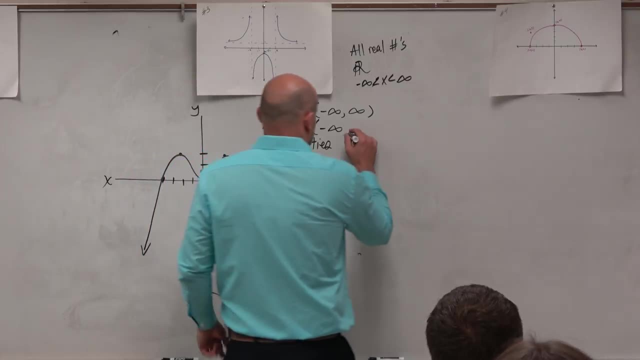 the way down. It's going down to negative infinity, But the graph continues as high up as 1,, 2,, 3, right, Yes, No. And 3 is contained. It's a part of the graph. It's a value on the graph. 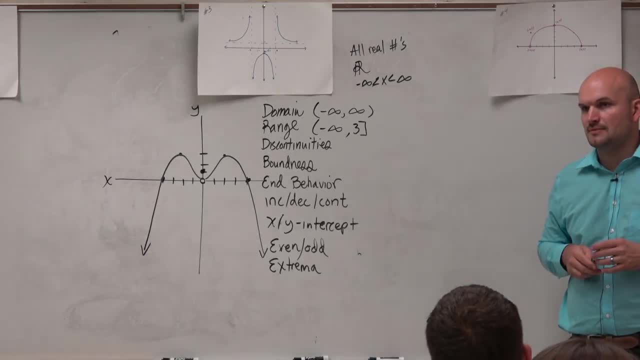 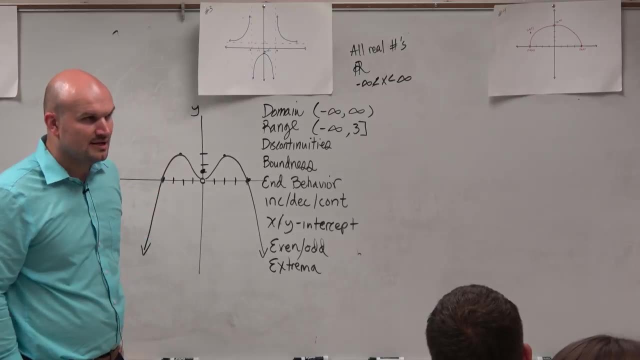 So, therefore, that's why we're going to use the bracket, All right. The next one is discontinuities, or we want to determine: is the graph continuous? And basically, guys, if the graph is continuous, that means we can draw it. 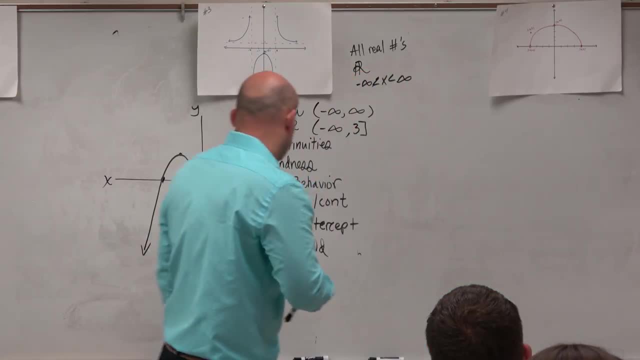 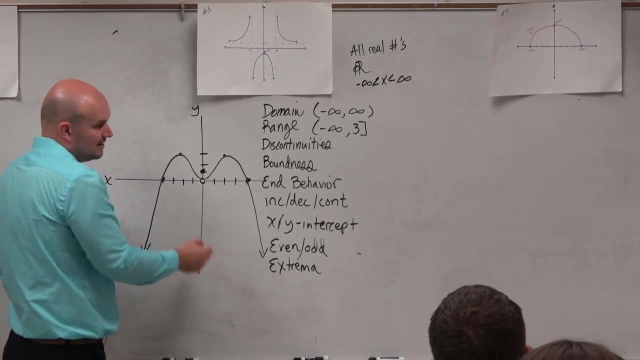 We can draw or trace the graph without lifting up our pen or pencil. So as you guys try to do that, you notice that we kind of come to a hole, that we have to skip over that hole to continue graphing Correct, And then we have to actually fill in that point. 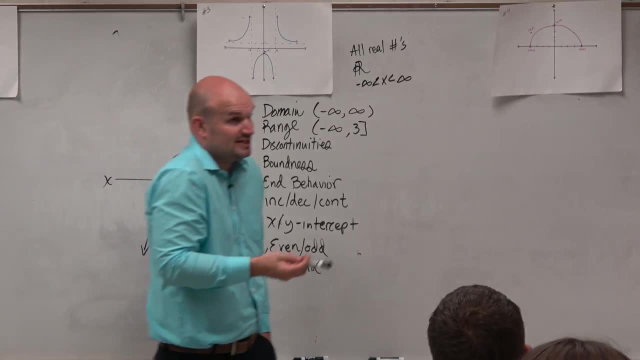 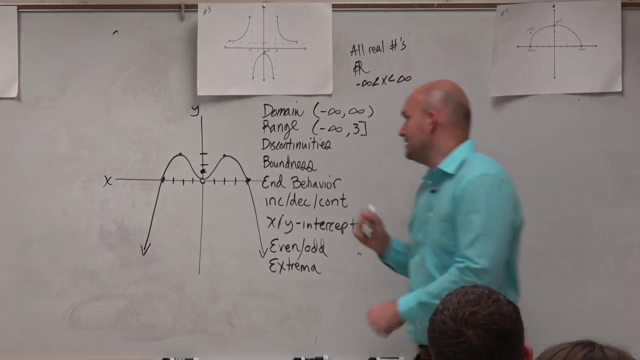 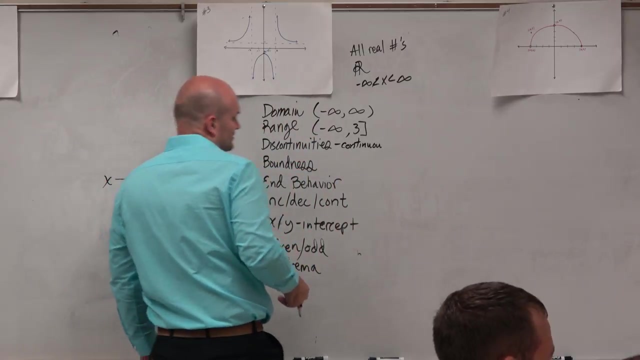 and then come back and do that. Yes, So it's non-continuous. It's only continuous if you can just nice graph it without lifting up your pen and pencil Now. so we would say it is continuous. I'm sorry, We would say it's discontinuous. 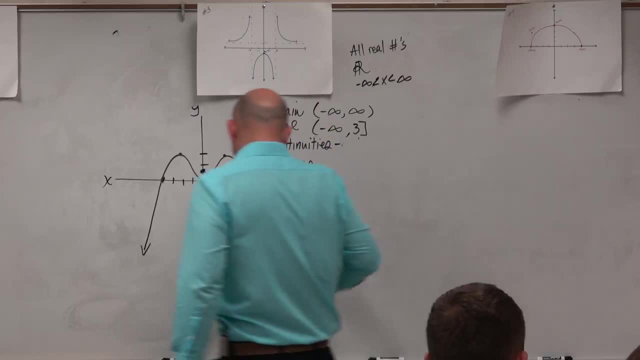 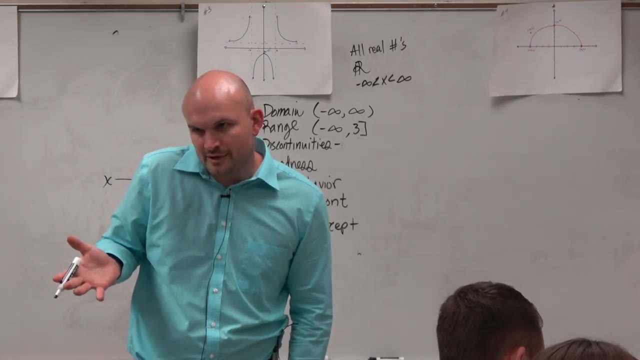 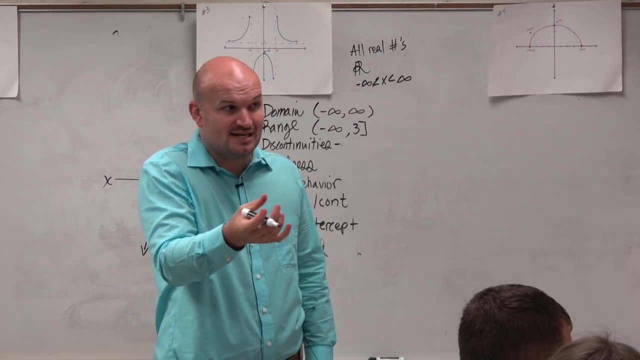 OK, But a lot of times the question is not going to say, oh, is it continuous or discontinuous? That's kind of obvious. More of the time we want to ask what type of discontinuity is there? If there is a discontinuity, what is there? 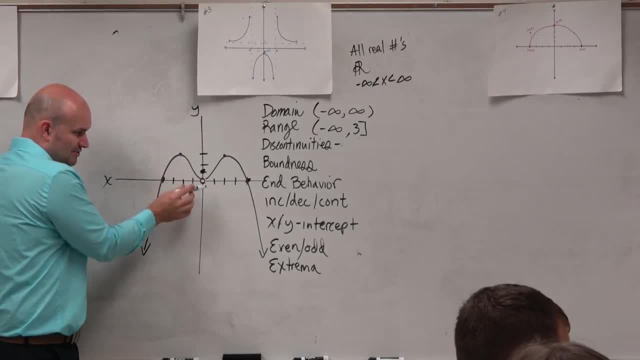 What type of discontinuity is there? So this, if you guys look in this graph, you can see this graph is perfectly OK, except there's a missing spot here, Right, And it's really just one value, One value that is undefined, which we call a hole. 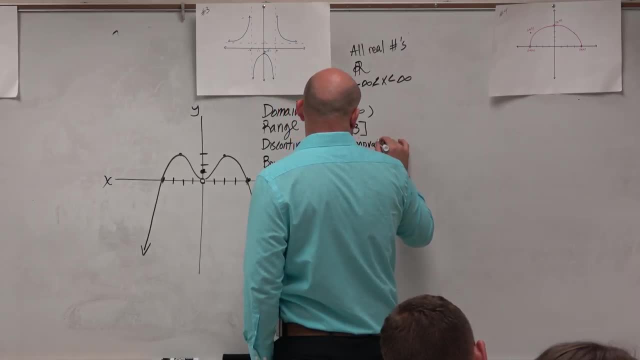 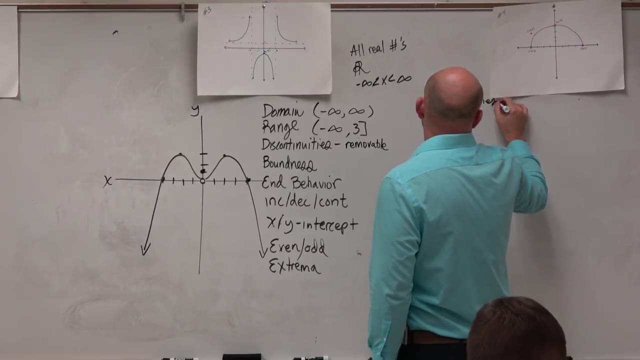 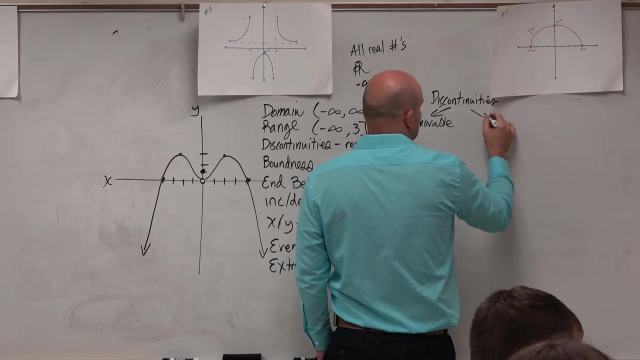 Now a hole is what we call a removable discontinuity. So I'm just going to put this over: When you're looking at discontinuities, you have removable and non-removable And, like I said, guys, this is like in your notes. 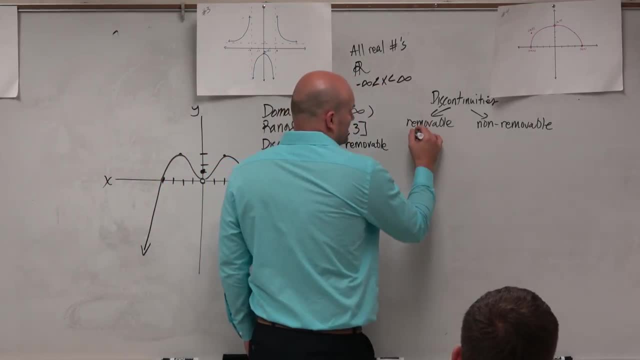 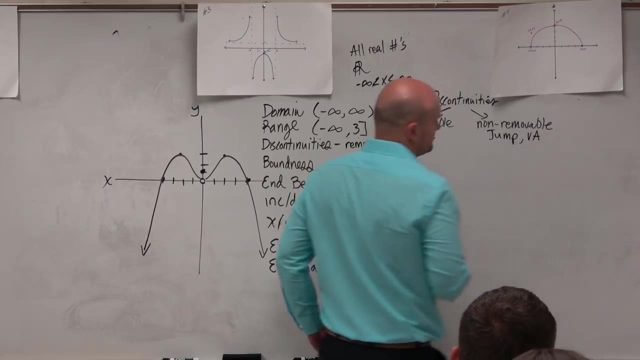 but it's just, I think, a good thing for you guys to remember. Removable is like a hole, Non-removable is like a jump or a vertical asymptote. So if you have a discontinuity, that's a vertical asymptote. 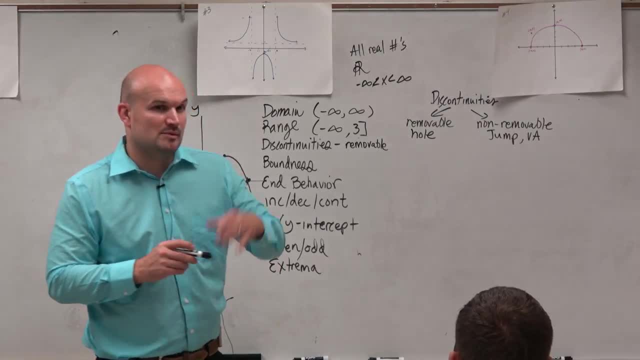 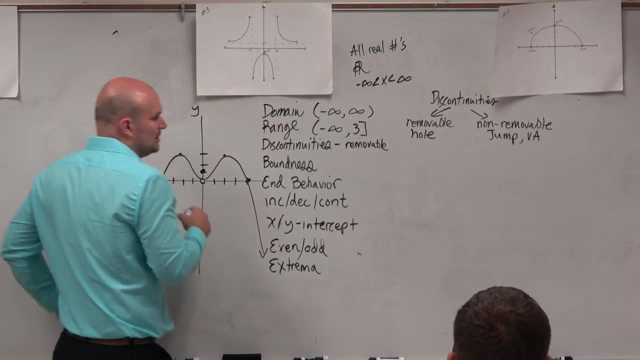 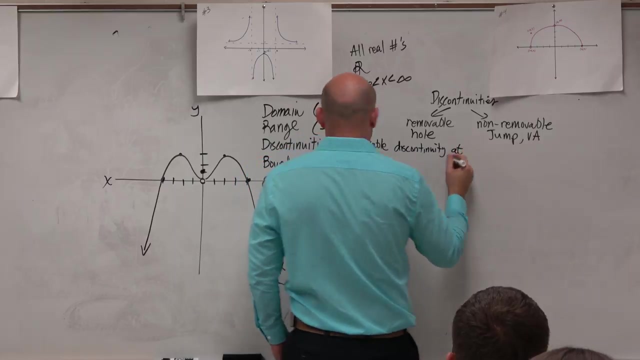 it's non-removable. And if it's a jump, which means you're going from one function to the next, that would be a non-removable as well. So we would say: this is a removable discontinuity. at say, x equals 0.. 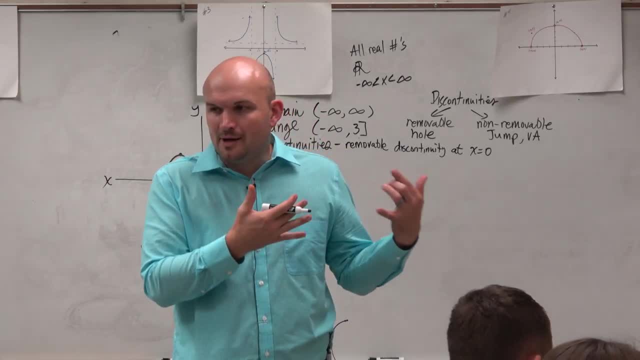 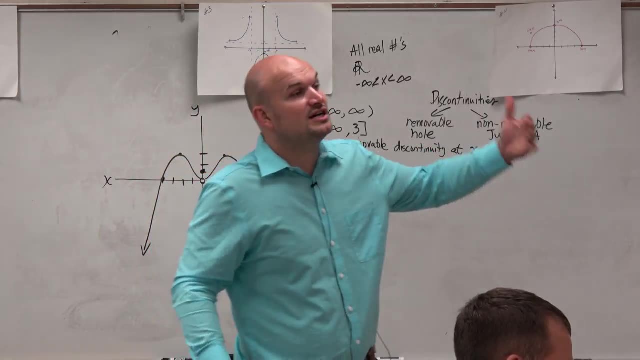 Now again it all kind of depends on the frame of the question. Up here in the problem I just say hey, continuous or discontinuity. So sometimes I might say, hey, label the discontinuities, Or where are there any discontinuities? 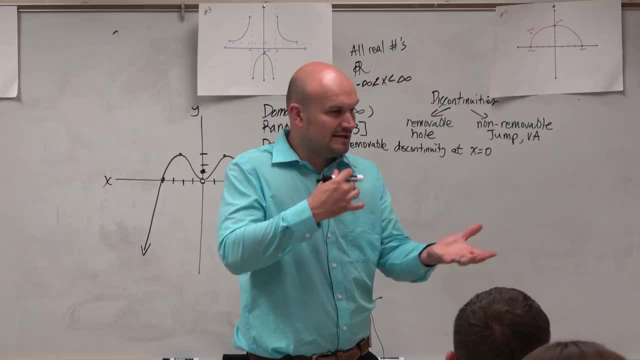 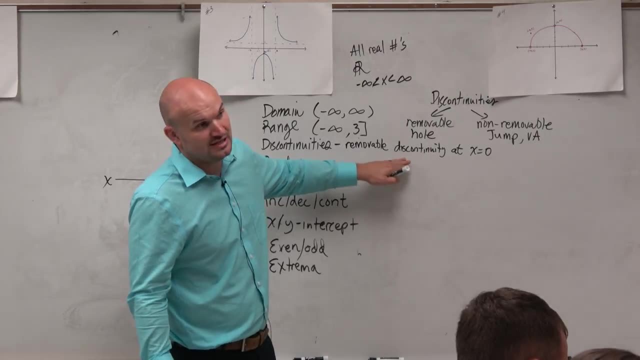 Or I might just say: is the graph continuous or not? So I mean there's a lot of different questions I can ask from you. The main thing I want you guys to understand is this is a removable discontinuity. So you could say it's a hole which is removable. 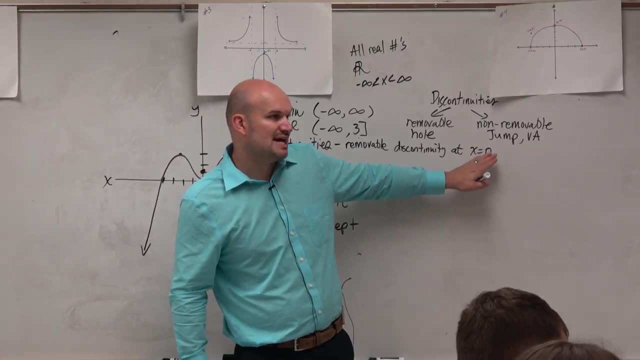 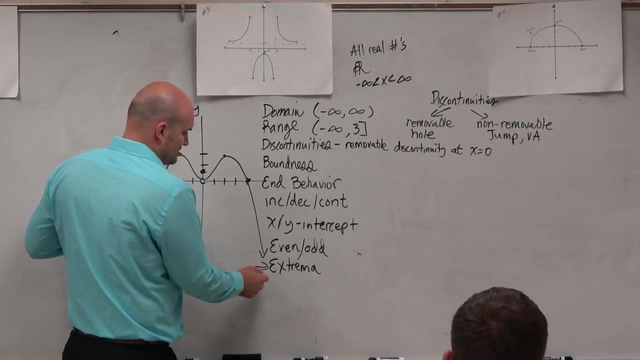 And there's a location of this discontinuity, which is the x value at 0.. I'm actually going to skip ahead to extrema, because extrema makes boundness make sense. So when we're looking at extrema, basically what we're- 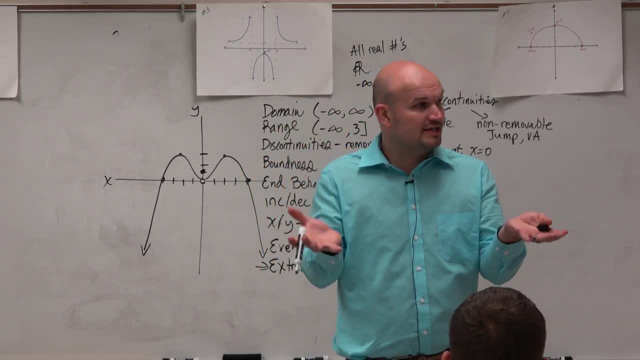 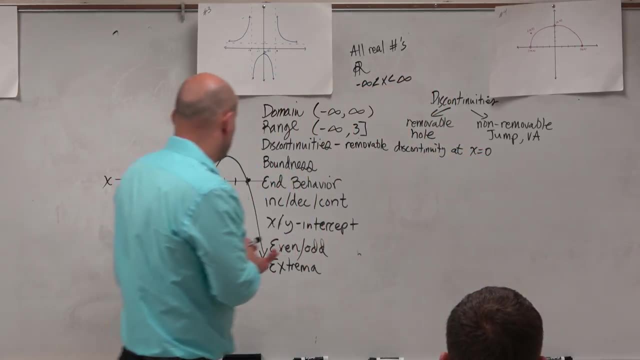 doing is we're looking at the maxes and the mins of the function. So we basically want to know: is there points that are highs and lows of the graph And you can look in here and we could say, oh, there looks like there's a couple. 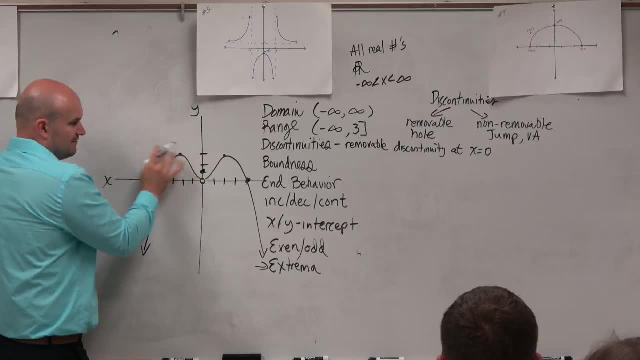 of different highs and lows. here Looks like, if you look at this, the graph only goes as high as these two points, Correct? And the other definition, or the best definition for maximums and minimums if you have a maximum point. 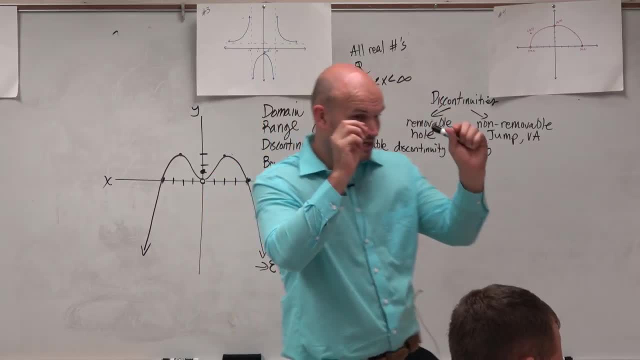 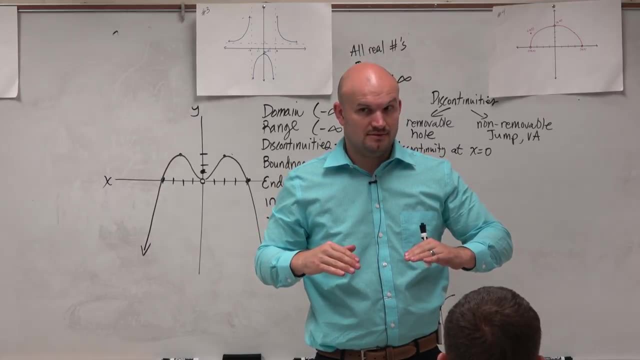 and this makes sense to you, or it should. If you have a maximum point, that means every point to the left and every point to the right should be below that point. Would that make sense? Yes, Any point to the left and any point to the right. 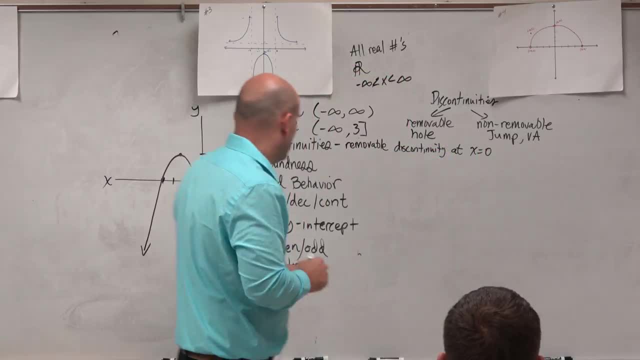 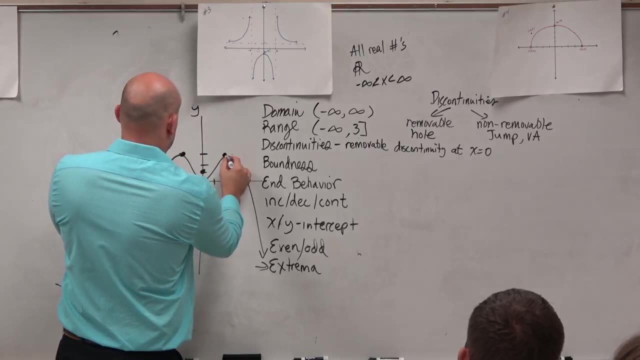 should be above that point, Correct. So if we kind of look at this graph, we kind of say, hmm, this is supposed to be a negative 2. If we look at these two points we kind of notice, hey, if I pick a point to the left and I pick a point to the right, 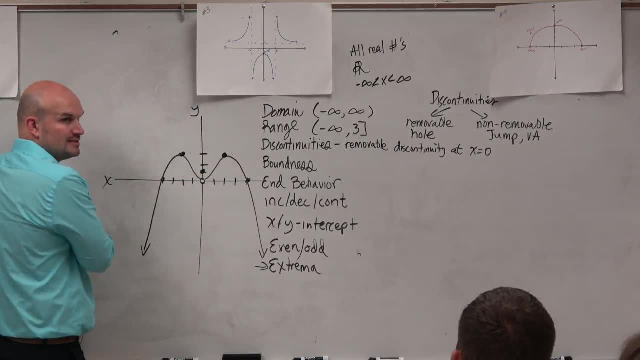 they're below this point, And that's true for this point as well. Now, not only are these the highest and the lowest points, these are the highest and the lowest points. These are the highest and lowest points of the function, Correct. 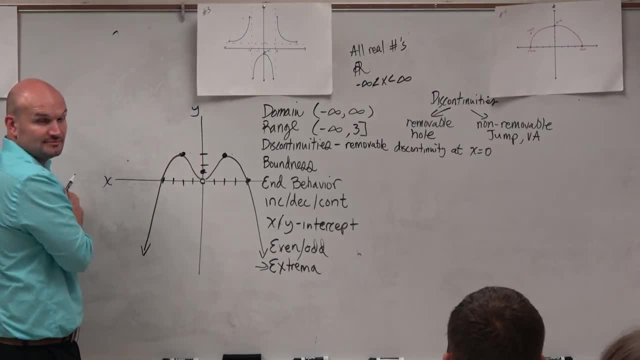 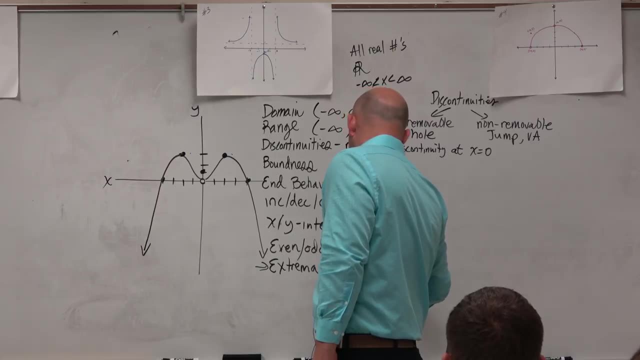 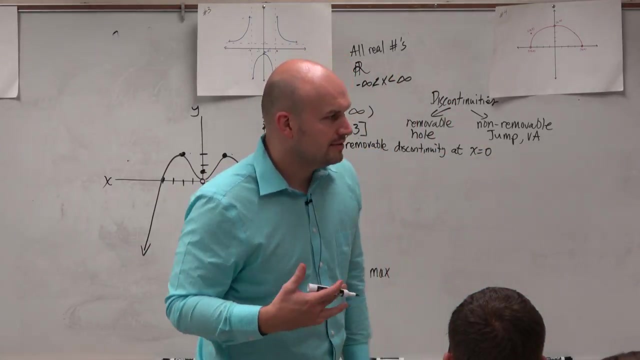 There is not one point that's even higher than this, Would you guys agree? So this extrema, these are what we call absolute extrema, Or we could just call them absolute max, So they're absolute maximum values. Now, there's a couple different ways. 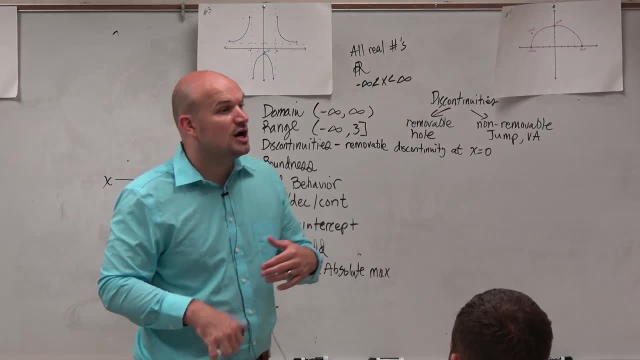 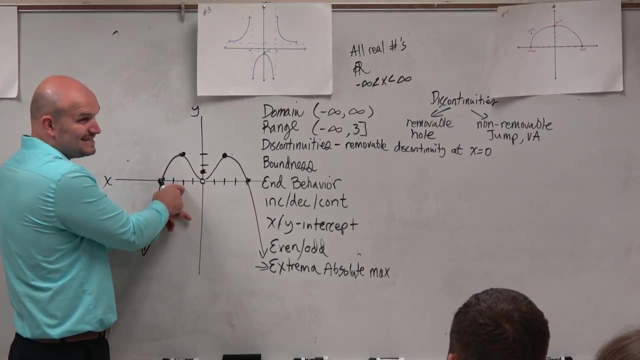 we can talk about absolute maximums. We could talk about absolute maximums of where they occur. Where do these occur? Where do these occur? Where do these absolute maximums occur? They occur at negative 2, at x equals negative 2,. 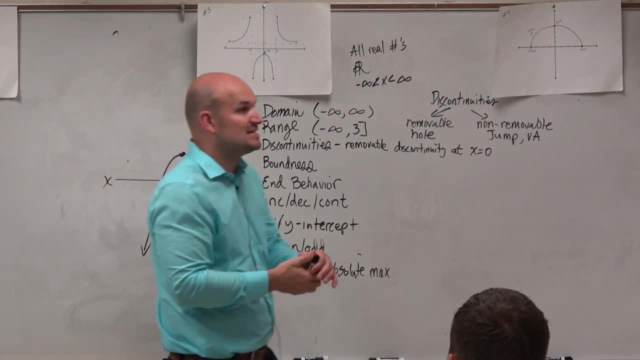 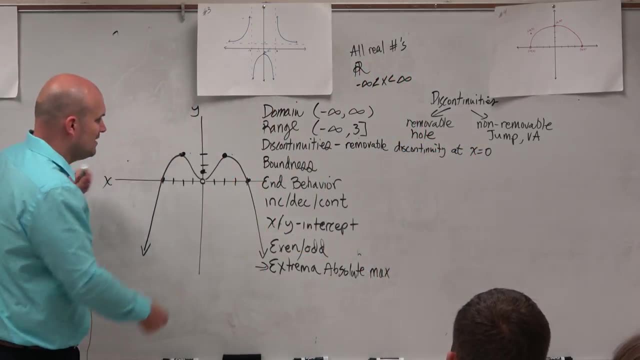 and at x equals positive 2. We could also talk about the maximum values. What are the maximum values? Well, the maximum value of this graph, the graph, does not go any higher than y equals 3.. So, when we're talking about extrema, 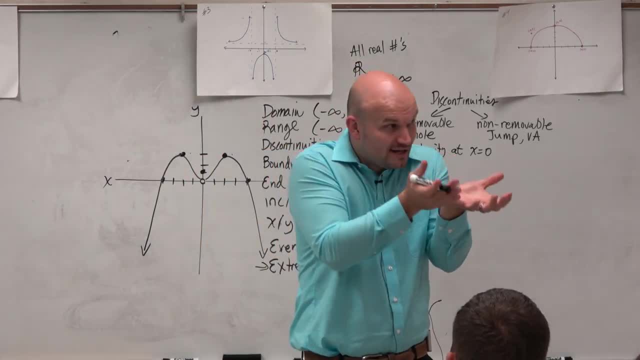 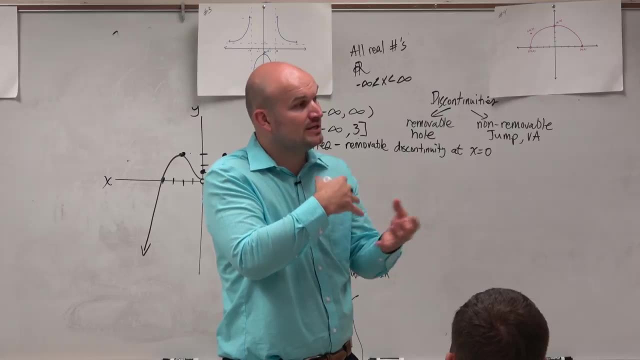 we can talk about where and what. Where is that maximum or minimum And what is the maximum or minimum? OK, Do you guys agree with that? So just be careful when you guys get to testing portions, Make sure you're answering the correct question. 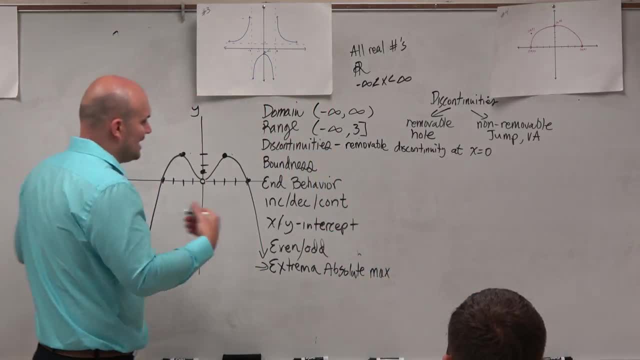 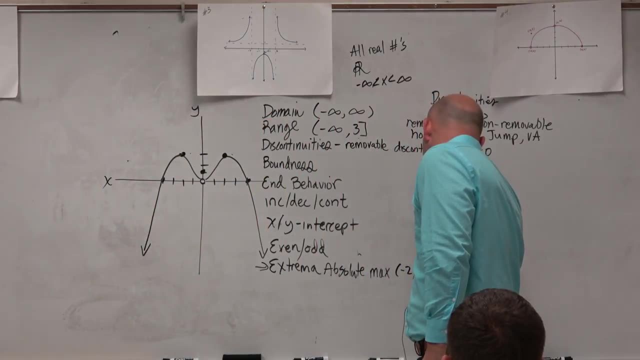 It might be where or it might be a what A lot of times you can get around that by just saying there's absolute maximums at negative 2, 3, and 2, 3.. So by giving the coordinate points, 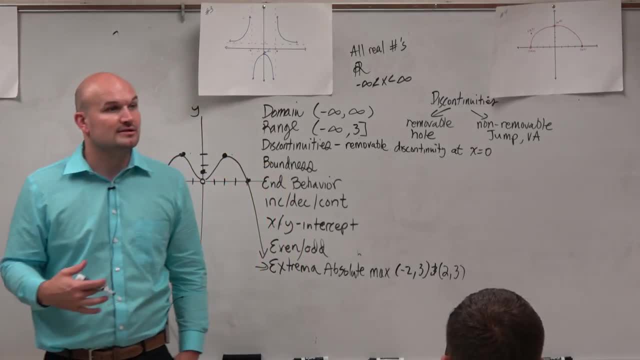 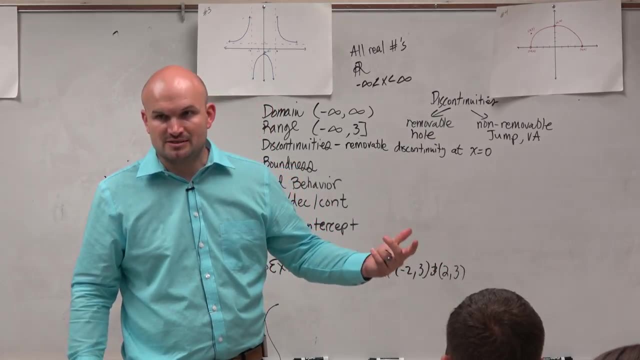 you are now providing a location and a value. You're saying the location occurs at the x value and the absolute maximum value It's 3.. And you can have more than one absolute maximum as long as it follows in that definition. 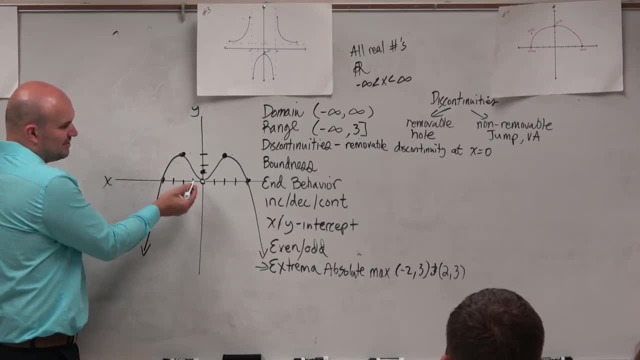 Now this one gets confusing. or this one looks good, Because wouldn't you guys agree that this looks like a point to the left and to the right? This should be a minimum right, But the problem is that's not actually a point. 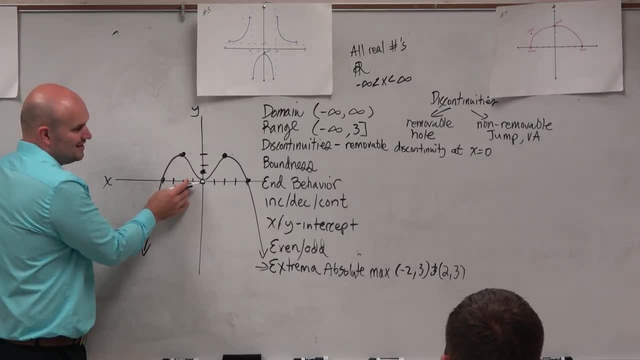 So you can't say 0, 0, because 0, 0 is undefined. Let's look at the point 0, 1.. If you look to the left of 0, 1 and to the right of 0, 1,, 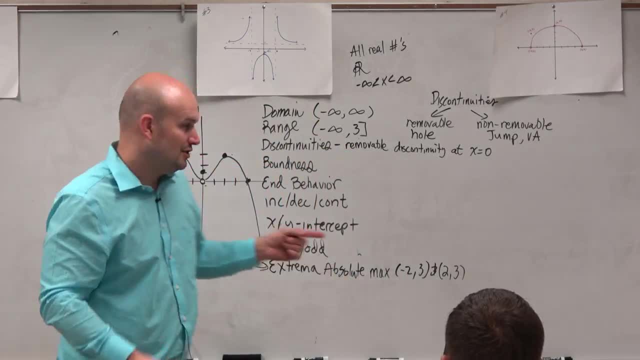 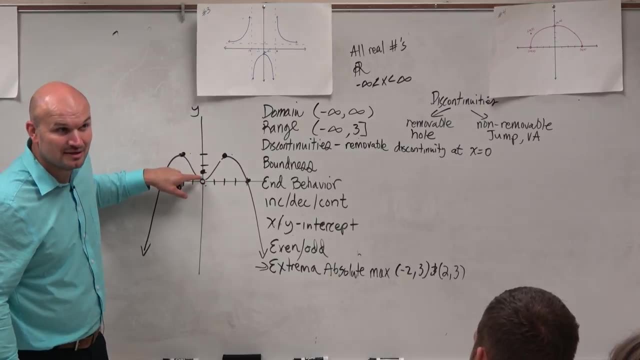 is that below 0, 1?? Look, look, you're not looking. If you go to the left or to the right, is that below 0, 1?? Yeah, So guess what? That's a maximum. Now, the difference here is all right. so you guys? 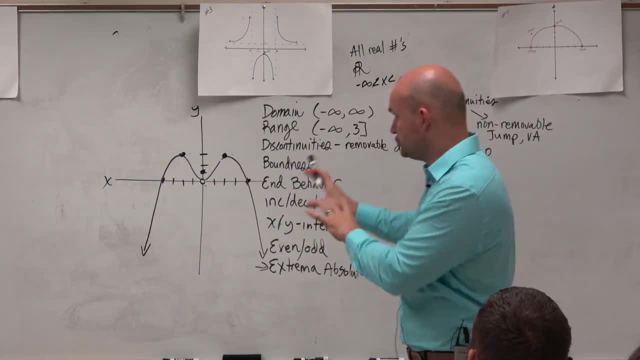 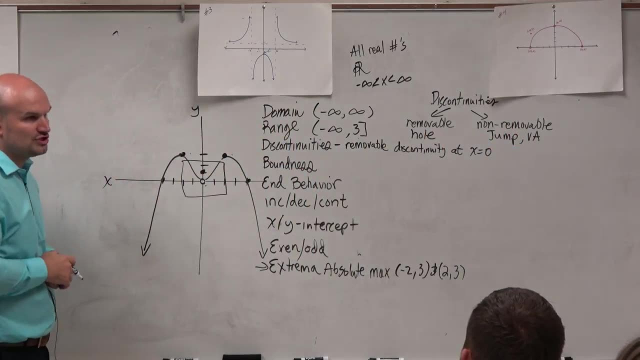 have my camera. right, If you take my camera and like: so we're zoomed out on this graph. Now, if we take my camera and we zoom in on this graph and we can only see that portion, does that look like a maximum? a well, actually. 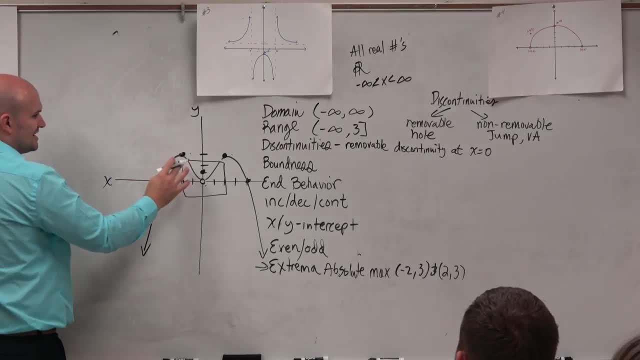 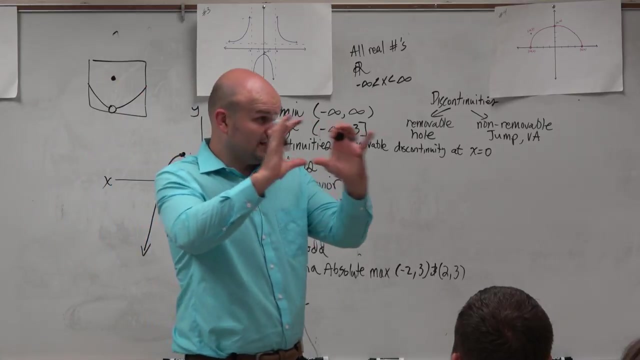 that's getting. let's get even closer. That's not a good zoom in. Let's get even closer. What about if we zoomed in? so all we saw was this: I'm really zooming in really far right. Is this point now more clearly a maximum? 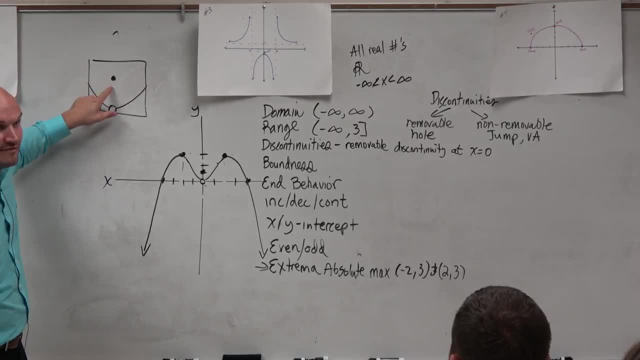 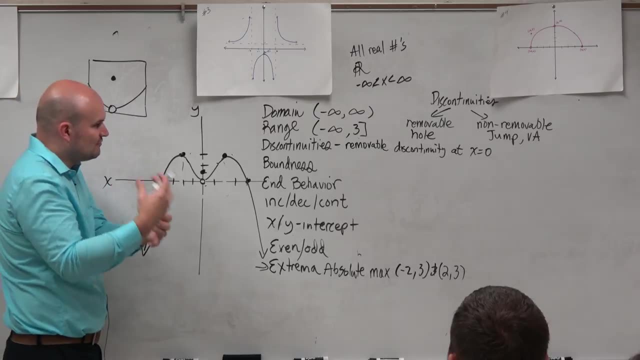 Is this now point? like? you can definitely see that that's a maximum point on the graph right, But as we zoom out we notice that there are values that are higher. So when we're talking about Maximums or minimums that are the highest of highs, 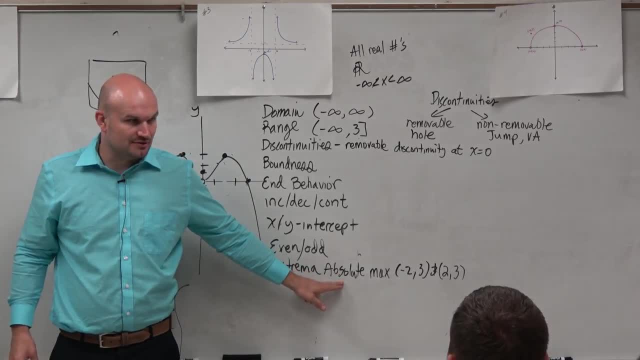 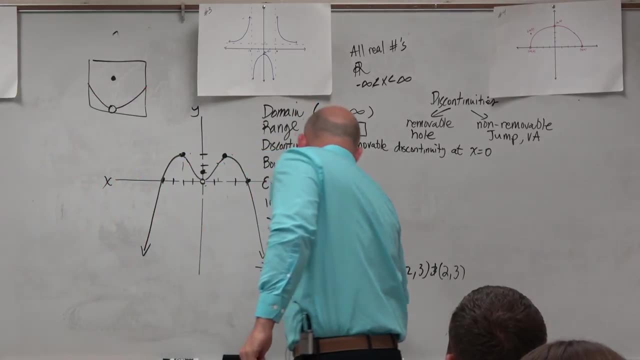 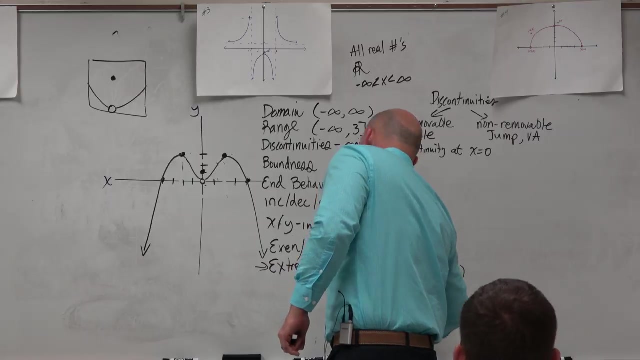 or the lowest of lows. that's where we use the word absolute. When we're just talking about a maximum, that's within a given range or interval, we call that relative, Or you could say local, And that's a relative max. So the relative max occurs at 0 comma 1.. 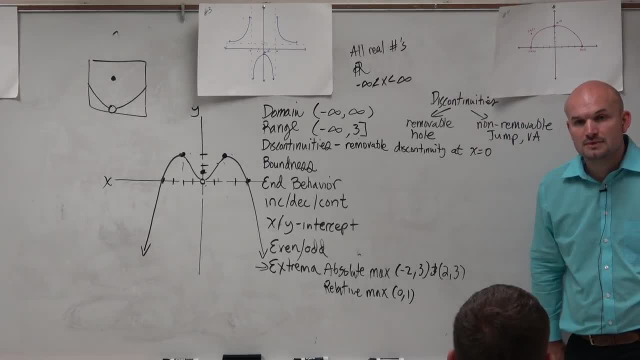 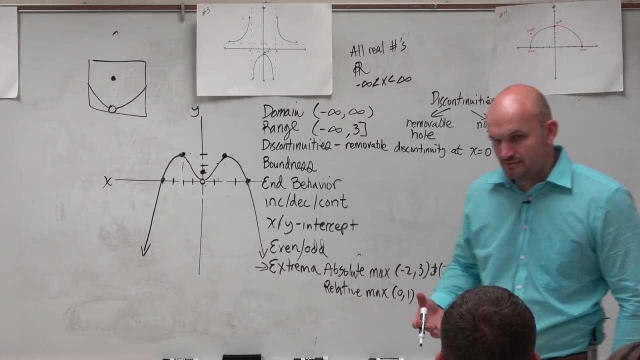 So then that's like the lowest max for his- Sorry- Is the minimum, as the lowest one there is The lowest. So if there is a minimum, then, but in this case we don't have any minimum values. There are no minimum values. 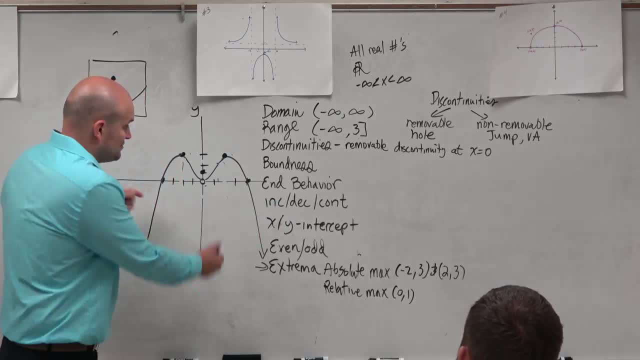 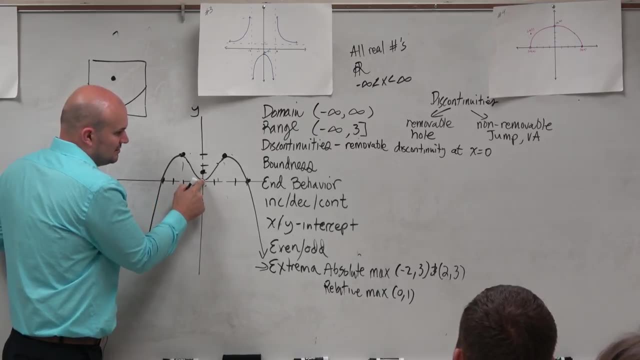 There's no point that represents a minimum right, Because if this was filled in then you could say 0, 0 was a relative minimum. But it's not filled in, It's open, And then obviously it continues down. 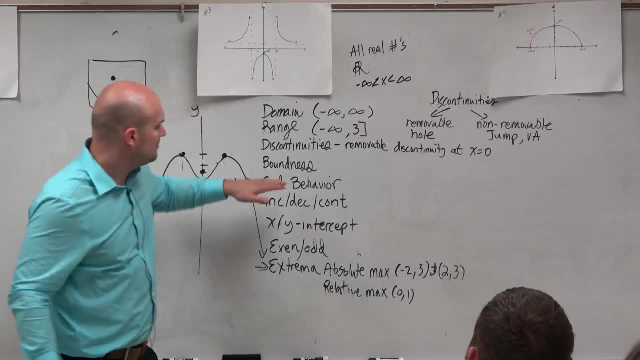 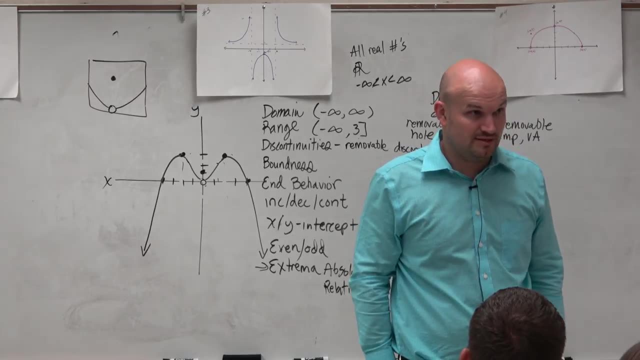 so it's never an absolute. OK. Now boundness comes in. Guys, if you get stuck with boundness, the best way I like to think about boundness is just replace boundness with restriction. OK, Basically, this is saying: where are 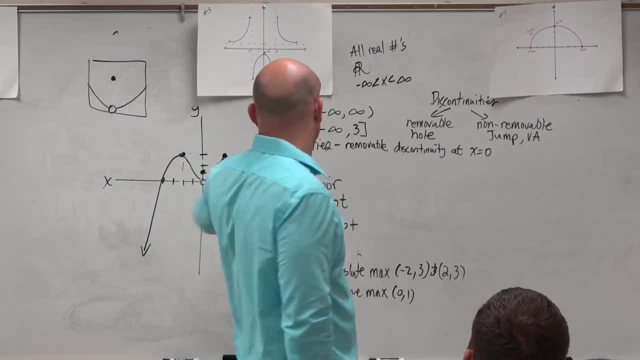 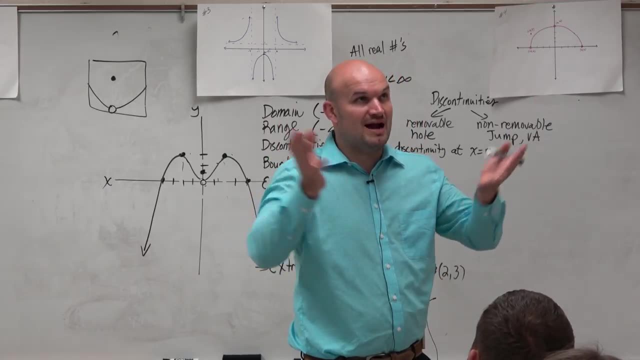 the restrictions on the graph. When we looked at nBehavior, I think only one group talked about nBehavior on their things. When you talk about nBehavior, you're basically saying the graph is continuing without bound or it's boundless. 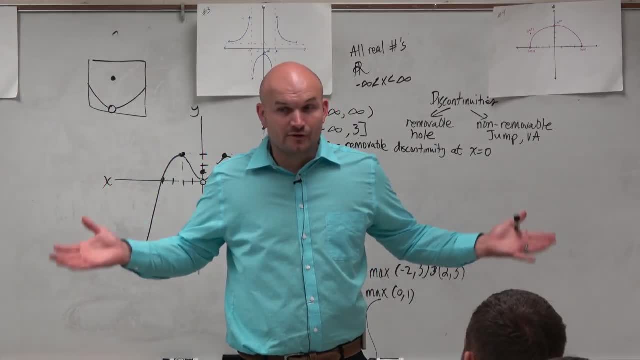 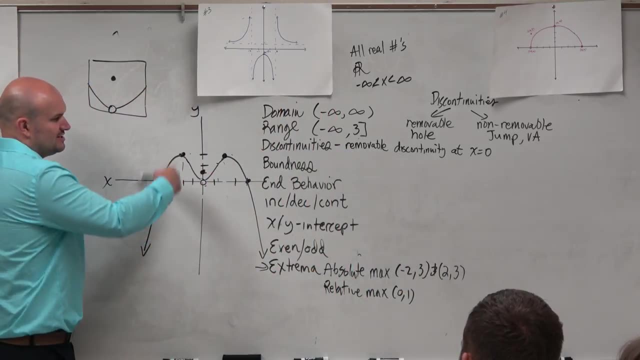 Think about the word bound and boundless. If something is continuing boundless, there's no restriction. There's no restrictions on it, correct, Like? look at this graph, Pretend it's like a roller coaster or something. As you continue on this roller coaster. 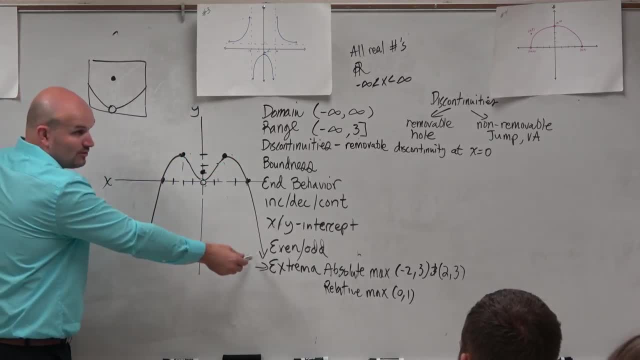 you're going down to infinity, right? There's no restrictions on how low you're going to go down. Does that make sense? So you are unbounded down here, You are unbounded below, But are you restricted on how high you can go? 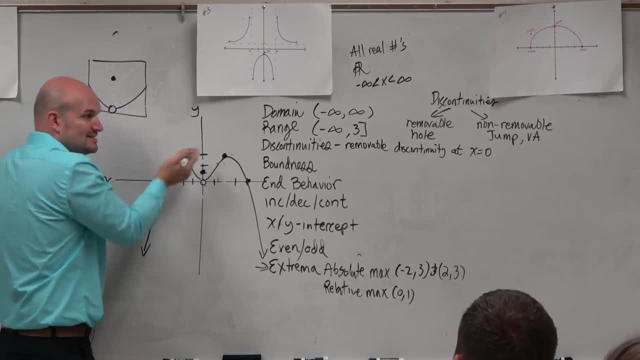 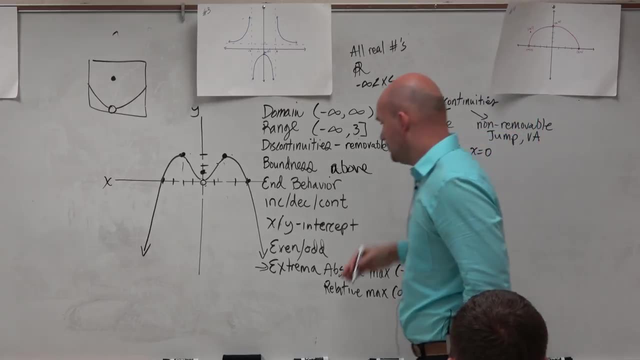 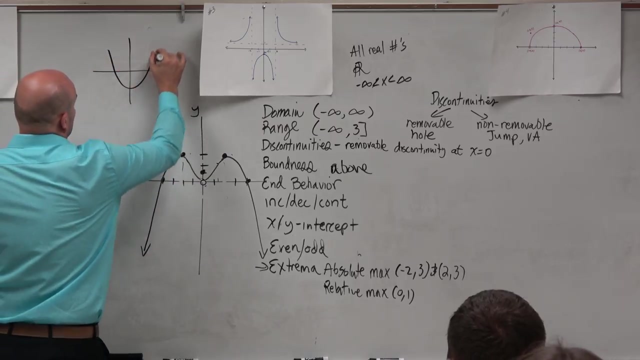 Yes, So you are bounded above or restricted above. So we just say abounded above And to give you guys a quick and easy definition here, or a quick and easy way to remember it, that's bounded above. That is an example of a function that's bounded below. 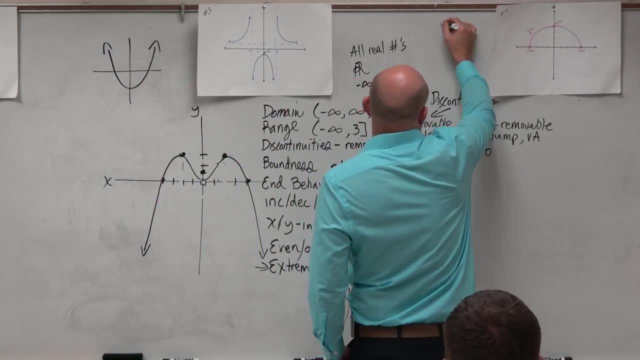 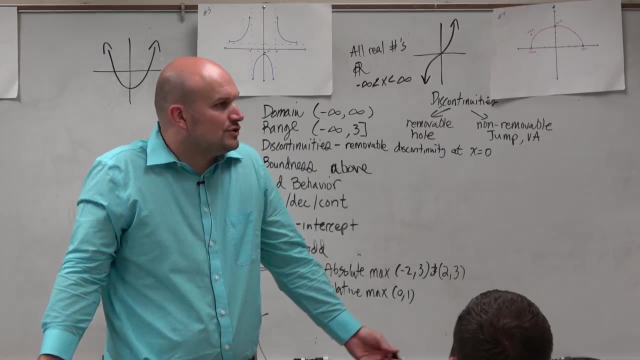 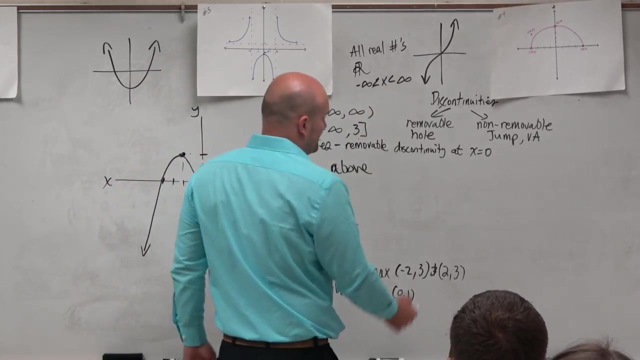 because it only goes at a certain value. If you guys want an example of unbounded, that function is unbounded because there's no restrictions- right, It's unrestricted. It continues indefinitely. It continues indefinitely in both directions, right. If you want something that's bounded top and bottom. 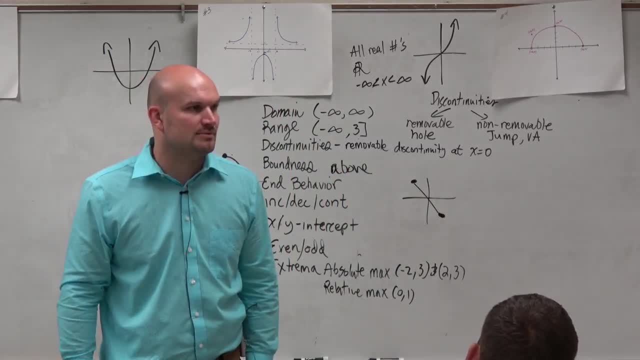 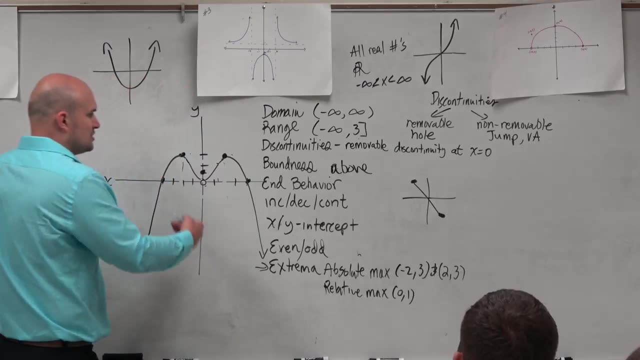 that's an example of something that's bounded, Bounded above and bounded below, because it's restricted on how high and how low it can go. Does that kind of make sense? So just look at your restriction. It's bounded, It can't go any high, so it's called bounded above. 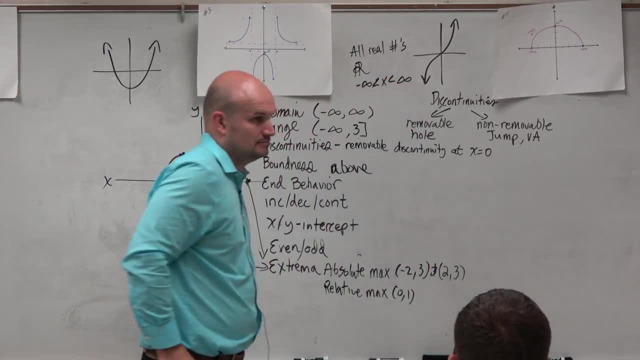 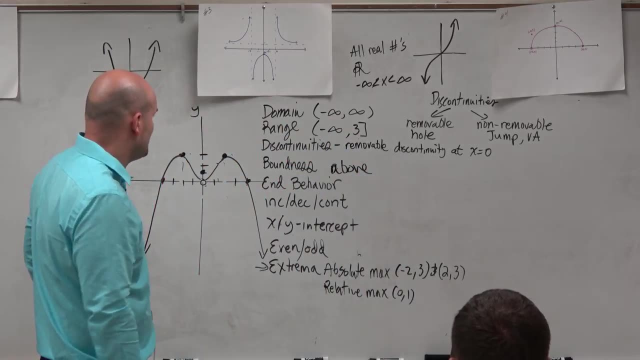 Yes, Wait. so bound is only it only applies to the end points. It doesn't like for like 0, 0, where it's like a bolt. that doesn't it? Yeah, we're just looking at the function in general. 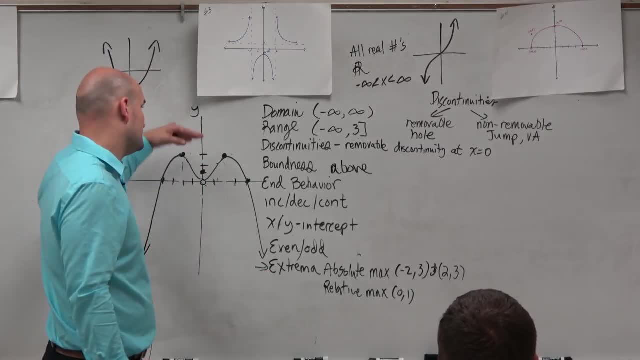 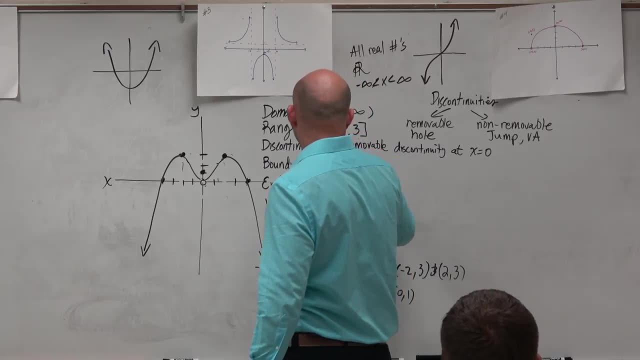 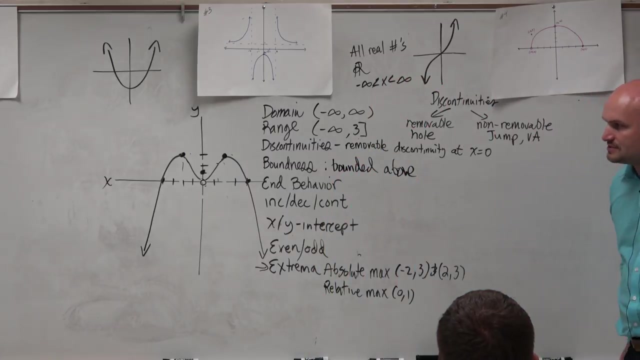 Is there a restriction on how high it goes or how low it goes? And if there is a restriction on how high, then we'd say it's bounded above, or we could say it's bounded above. The next one is end behavior, And so end behavior. we're going to spend a lot more time. 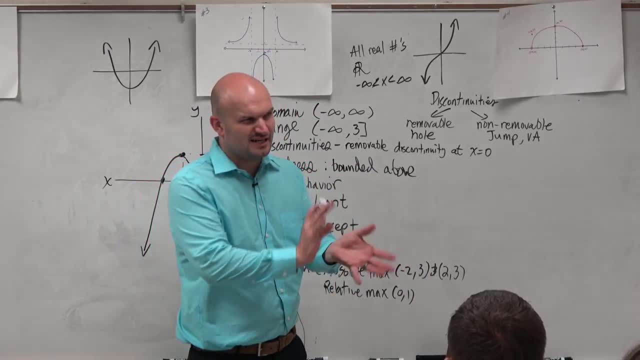 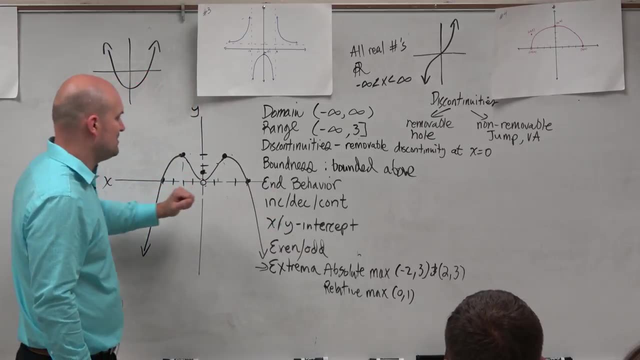 on this once we get into polynomials. So all I really care for you guys. there's a lot of different notations that we're going to talk about For right now. non-mathematical is perfectly fine. All I want you guys to all we're asking for end behavior. 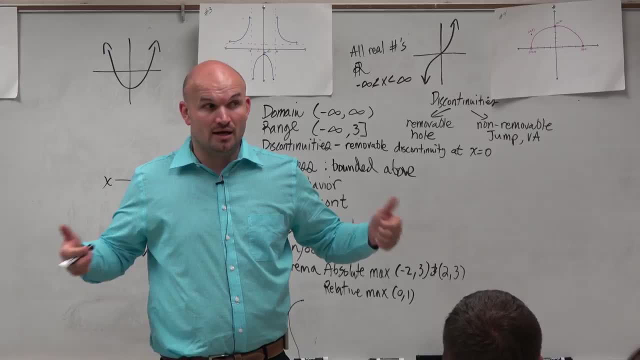 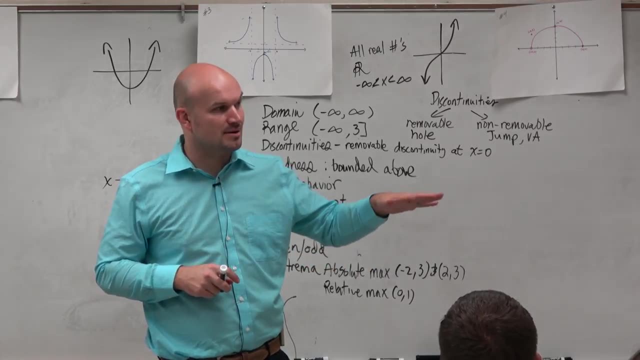 is as the graph continues to the right and to the left. where is it going? Up or down? Or be careful, it doesn't always have to be going up or down. It could actually approach a number or it could stop. 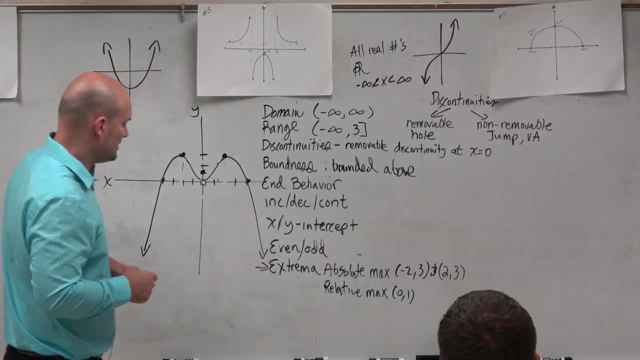 And therefore there'd be no end behavior OK. But in this case we have a pretty nice function here: This graph: as we continue to the left, the graph is going down. Usually we'll say false, Falling, or at least I prefer to say falling. 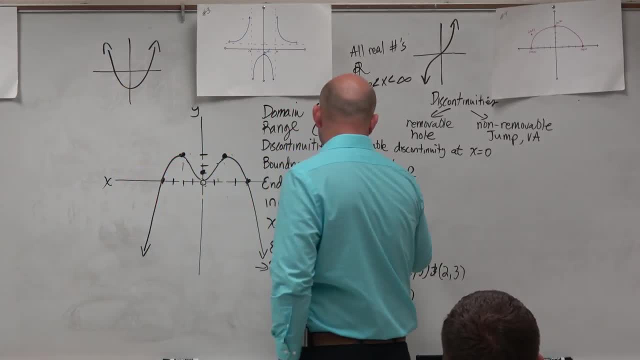 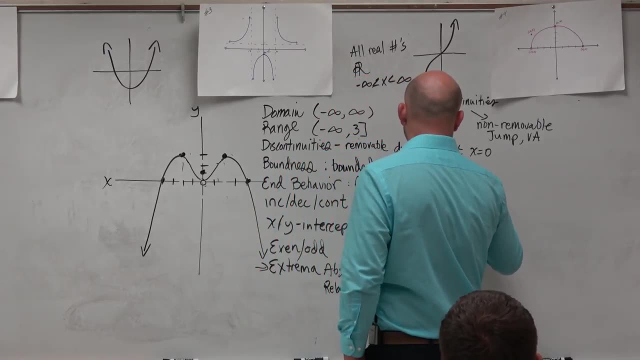 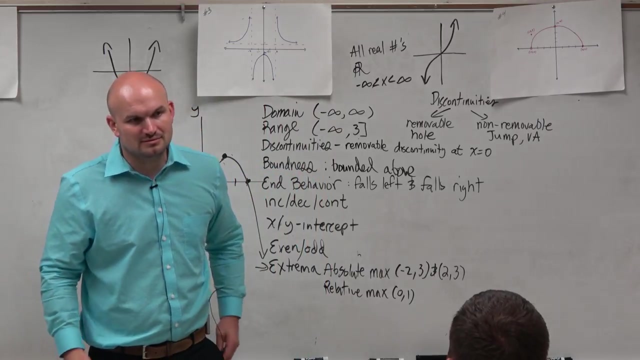 As we go to the right, the graph is falling, So we could just say I prefer falls left and falls right. That's a little bit more descriptive than down, down, up up, positive, positive, negative, negative, And don't worry. 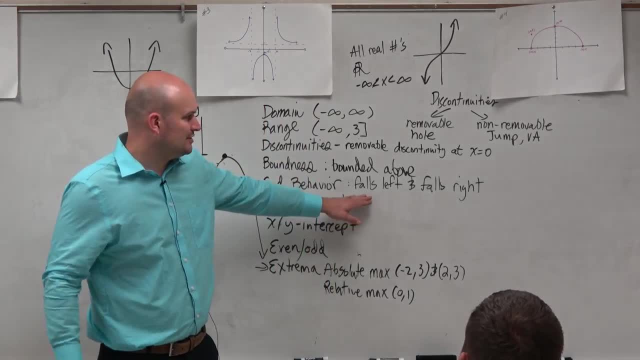 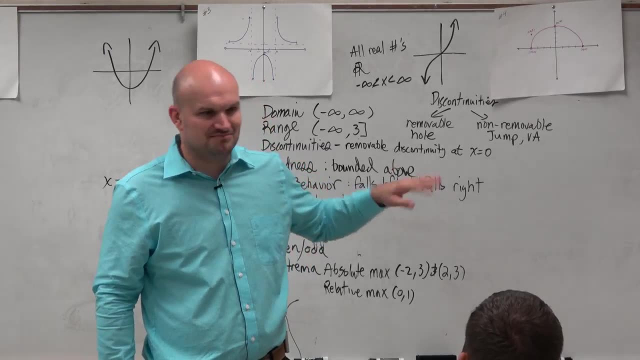 Yeah, I mean it's. don't worry, I don't really care too much about this, because next unit we're going to have a formal definition for end behavior, So the falling positive is not really going to. we're going to have a mathematical definition. 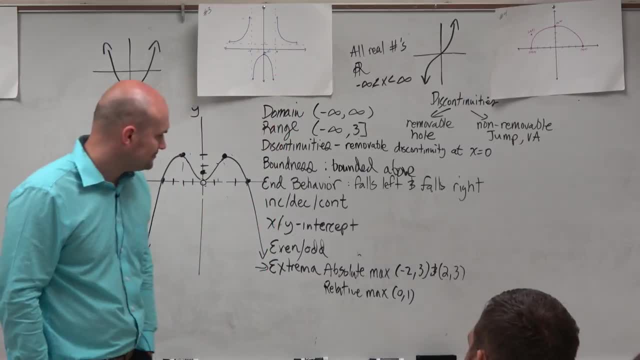 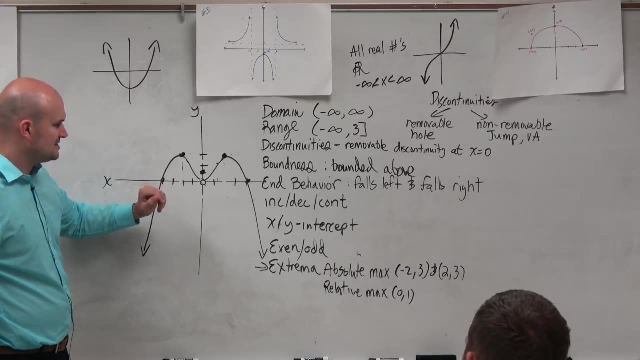 All right, Increasing, decreasing and constant. So actually let's do x and y-intercept real quick and even or odd, And then I'll do increasing, decreasing constant, So the x and y-intercept. you can see that here. 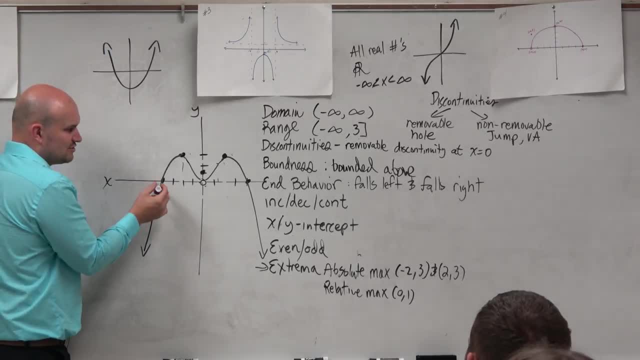 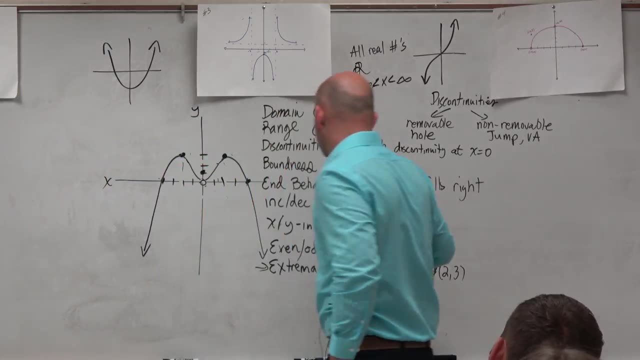 it looks like it, but there's no x-intercept, So you can see that it's crossing at negative 1, 2, 3, 4.. 1, 2, 3, 4.. So the x-intercepts, you could say at x equals negative 4,. 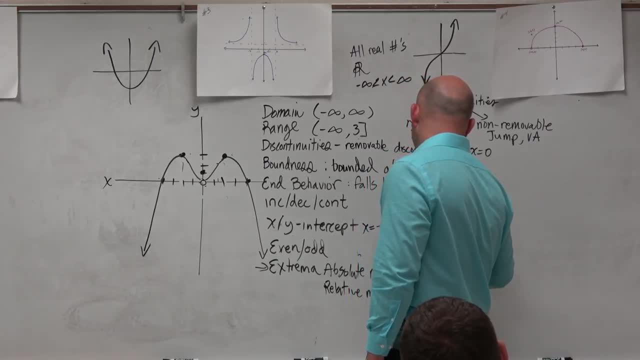 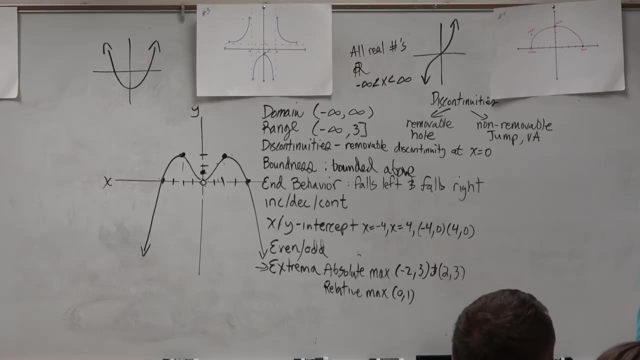 or x equals 4.. You could also write them, ladies and gentlemen, as coordinate points, which is my preferred method And the reason why I like writing them as preferred method, because it reminds my brain that when x is equal to negative 4, y is equal to 0. 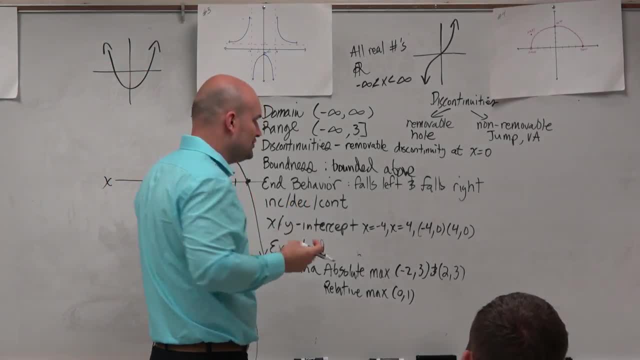 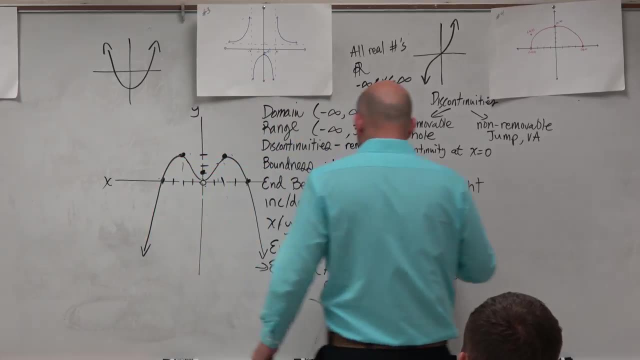 And that is very, very important later in this whole unit of understanding the intercepts, y is equal to 0.. 0 for the x-intercepts, And if I wanted to find the y-intercept, we just look at where the graph is crossing. 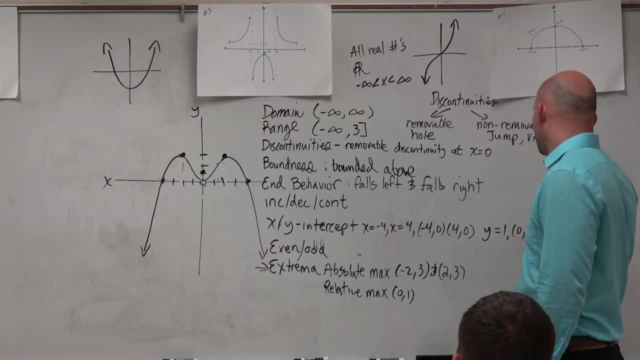 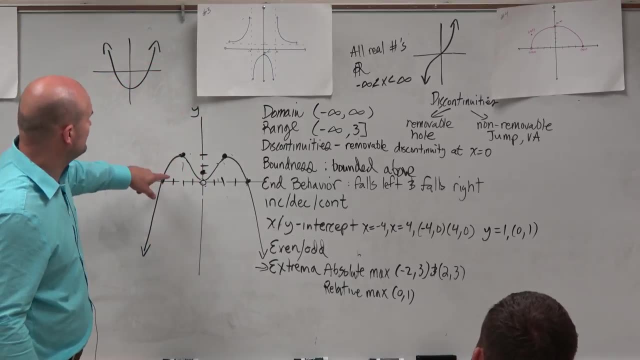 And you could say: the y-intercept is at y equals 1 or 0, 1.. So the y-intercept is when x is equal to 0.. Train it in my brain. Guess what? If something is symmetrical about the y-axis, it's even. 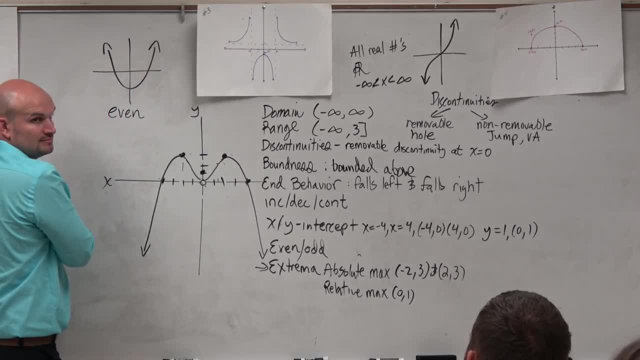 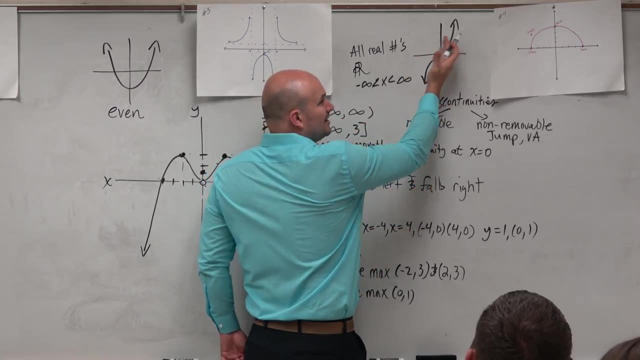 Everything to the left of the y-axis is equal to everything to the right. So it's, even If something is symmetrical about the origin. you've got to kind of follow me on this one, If you flip it about the y and then flip it about the x. 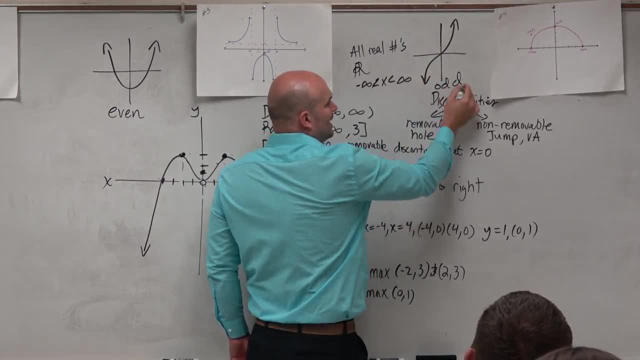 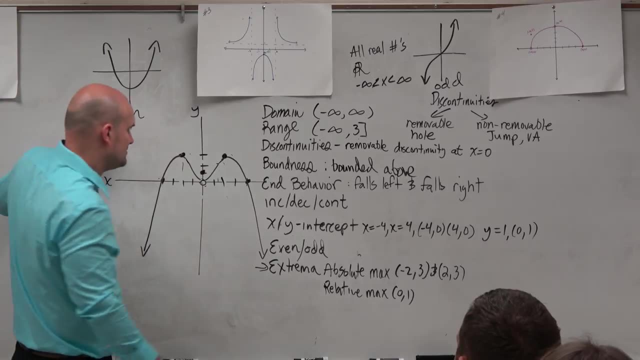 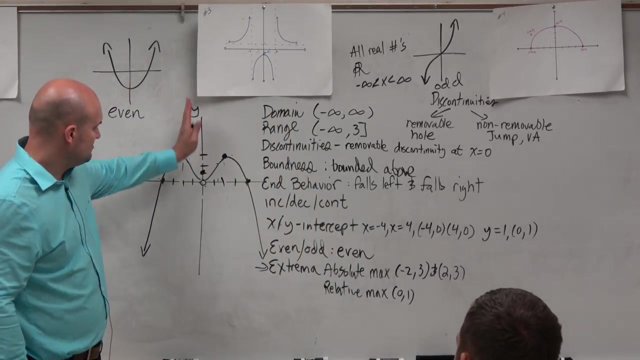 you get the exact same function back. So that's called add. And if you guys look at this graph, you guys will see that this graph has symmetry about the y-axis. So therefore it is even if it's symmetrical about the y-axis. 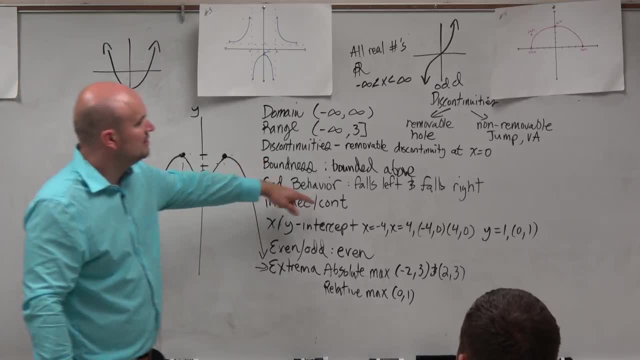 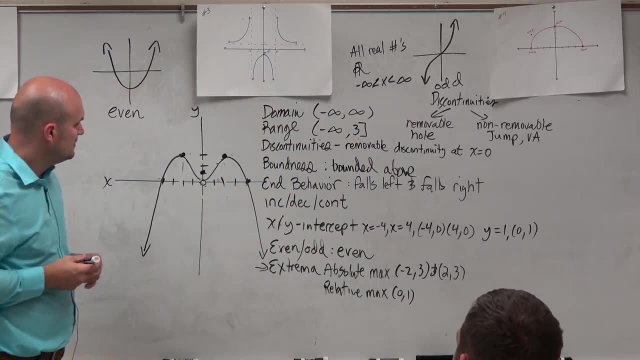 Everything to the left of the y-axis is equal to everything to the right. But if it's symmetrical about the origin, that means you can flip it around the x and the y-axis and it gives you the same function. All right, increasing, decreasing, continuous value. 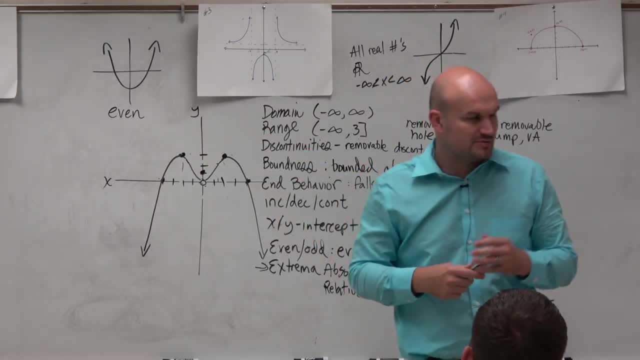 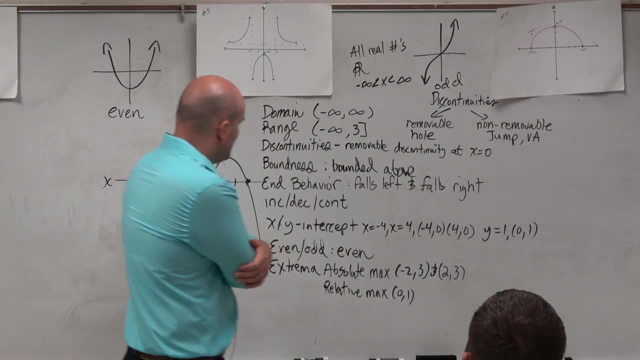 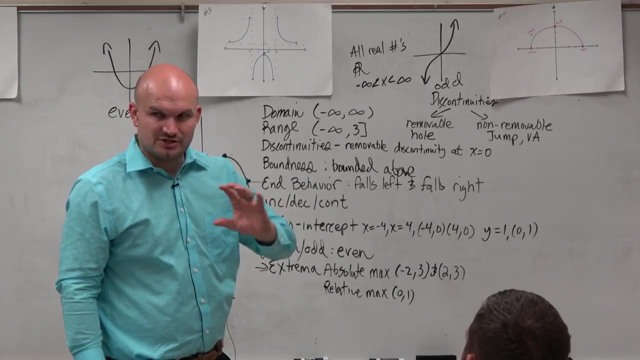 So this one gets pretty confusing And I think reading the last group's description kind of helped out with that. So when we're doing increasing decreasing values, everybody usually has a different take on this, And I want you guys to kind of understand this. 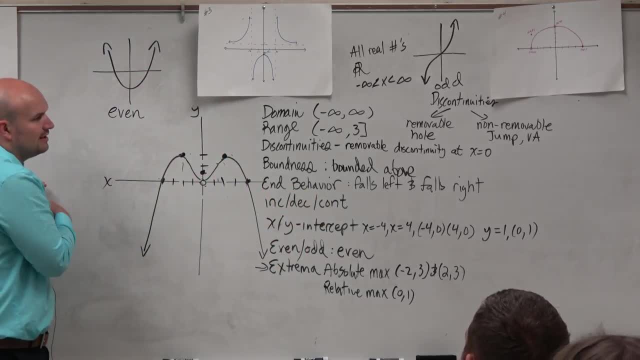 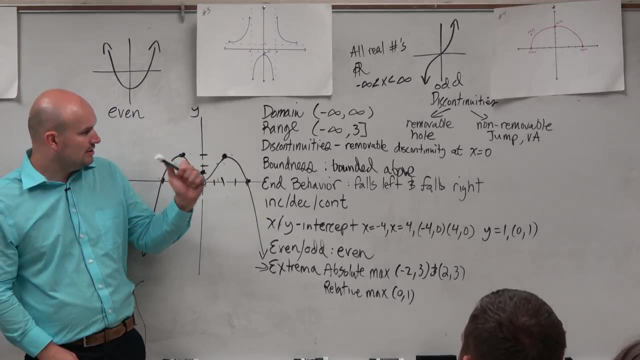 I want you guys to understand something If I'm describing this graph. there's a couple ways we could talk about this. We could say: how is the graph? increasing, decreasing or continuous? So let's actually look at the interval from 0 to 1, 2.. 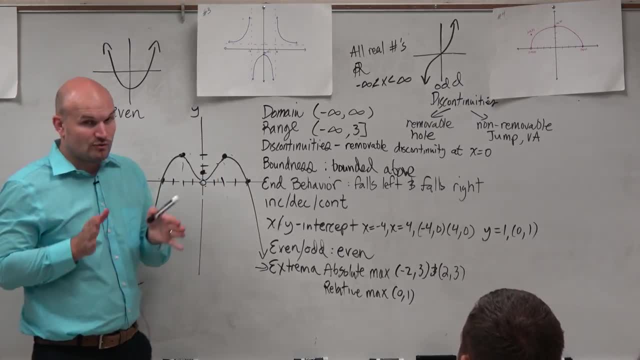 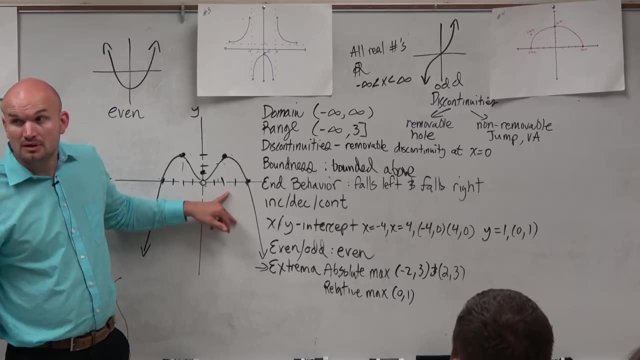 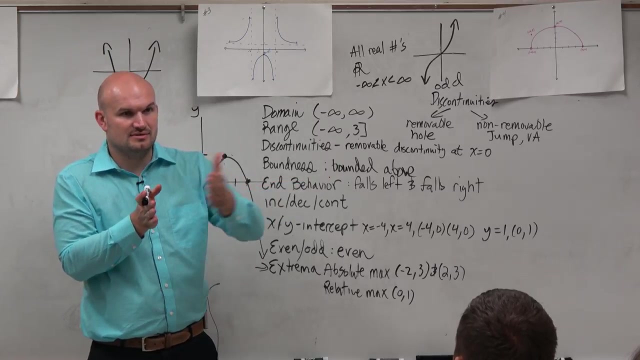 So from 0 to 2, right, I could say the graph is increasing from x equals 0 to x equals 2.. Yes, Does that make sense? So if I'm talking about location, I would want to use the x values, right. 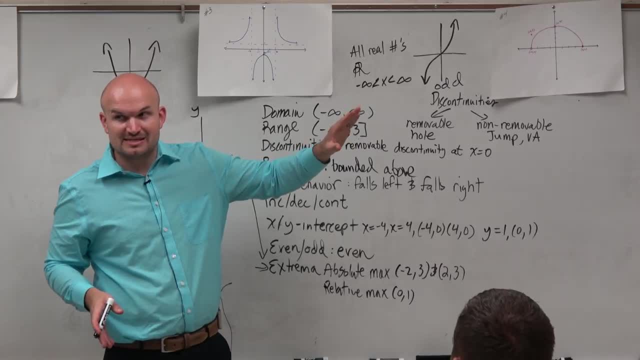 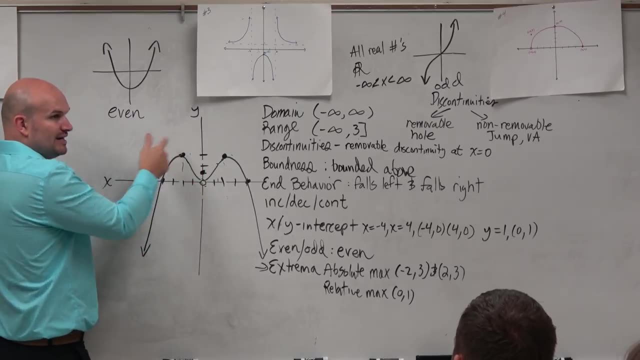 I'm saying from x equals 0 to x equals 2, the graph is going up. Does that make sense? If I say the graph is increasing from y equals 0 to y equals 3, that's basically giving me the values of how high it's. 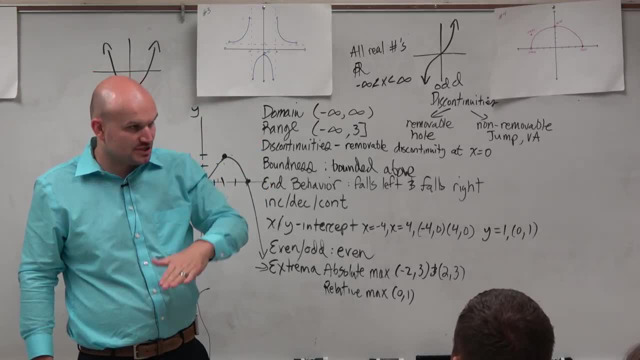 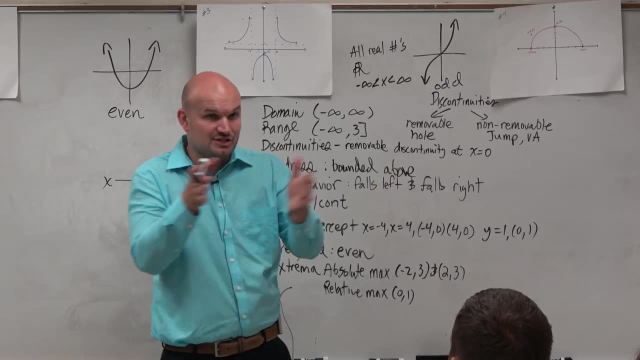 increasing and how high it's increasing from one interval to the next. Does that make sense? All right, So if you're talking about x values, you're kind of talking about location and y values, Right, You're kind of talking about the value of how high or low. 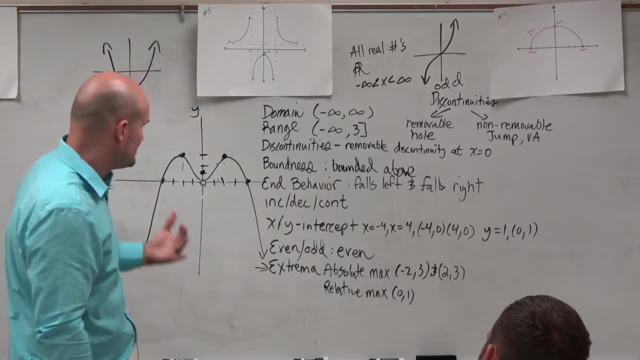 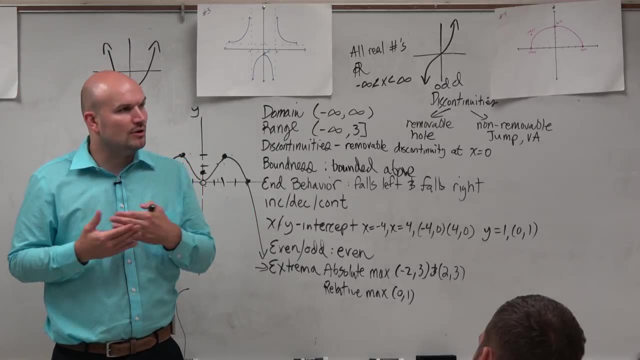 it's going Right. So when we are describing something as increasing, decreasing or constants, we only want to talk about when is the graph going up down, or when is the graph going up down or staying, remaining constant. 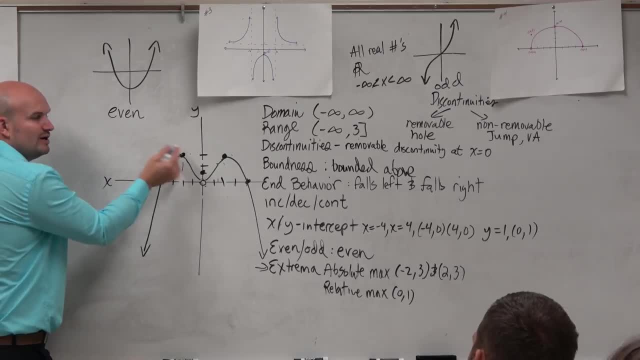 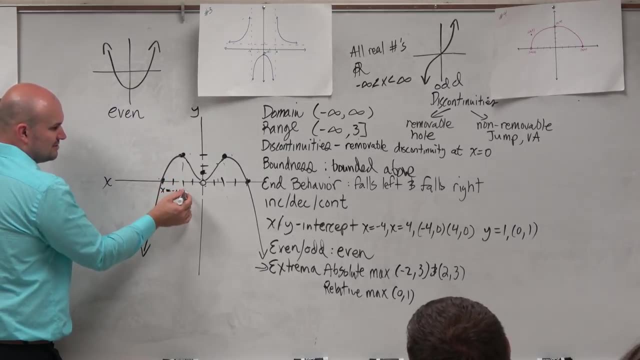 So what that means is, even though these have coordinate points, we don't care about the y values here. I don't 1,, 2,, 3, 4.. I am not going to use the y values, I'm just going to use the y values here. 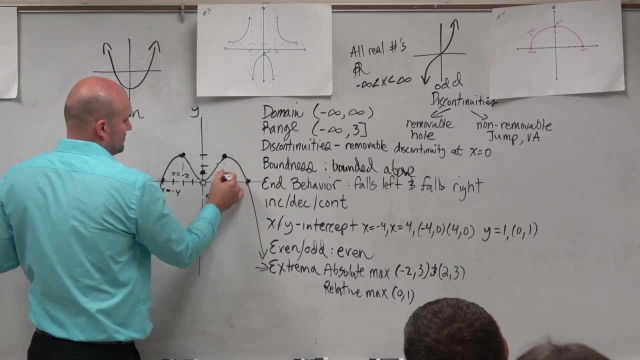 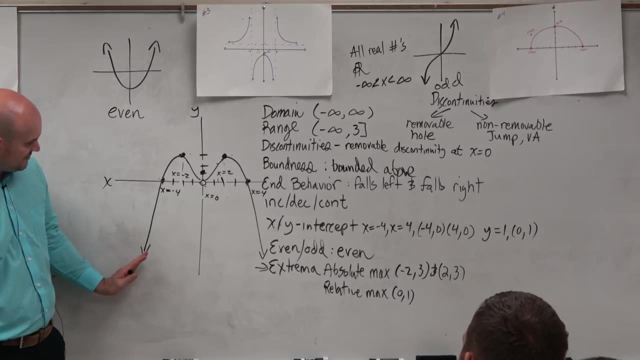 So when I talk about when is the graph increasing, I say: well, it looks like the graph starts from negative infinity to negative 2.. I don't need four of these: From negative infinity to negative 2, the graph is increasing. 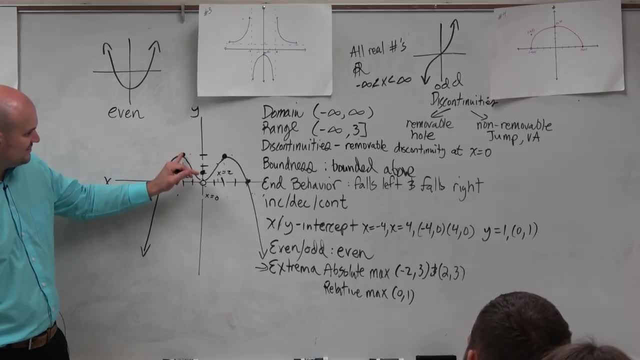 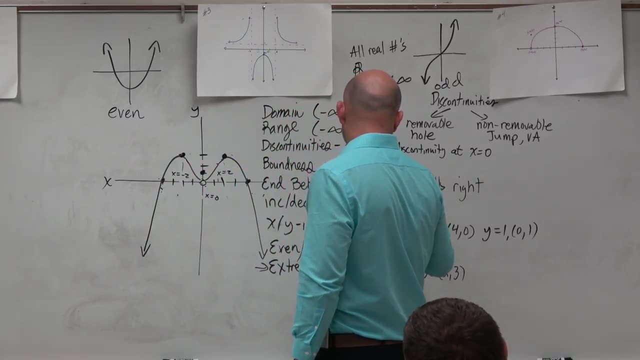 Don't you guys agree? So I'm going to say my increasing value is from negative infinity to negative 2.. So I'm going to say my increasing value is from negative infinity to negative 2.. Then does the graph continue? Does the graph increase on any other interval? 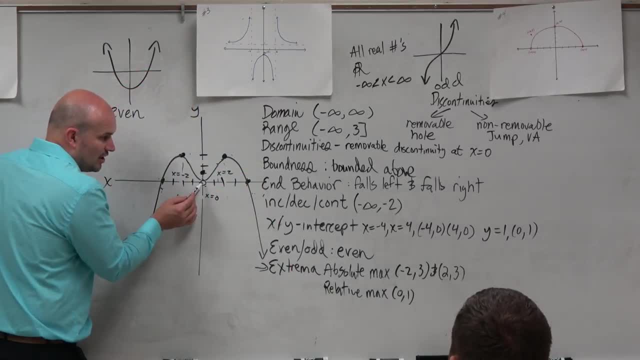 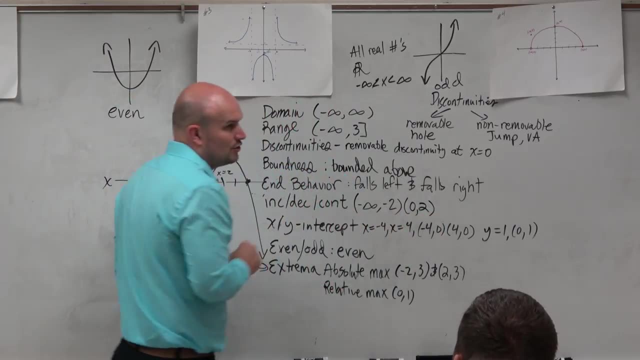 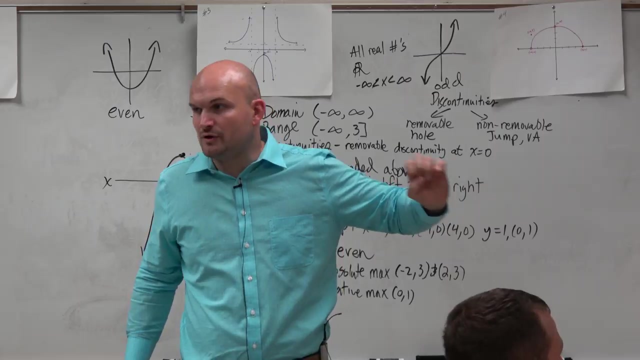 Is it going up or down on another interval? Yeah, from 0 to 2.. Now what I want you guys to understand: these are not coordinate points. If you guys look at my definition on the board, it says when is the graph going up, down or constant? 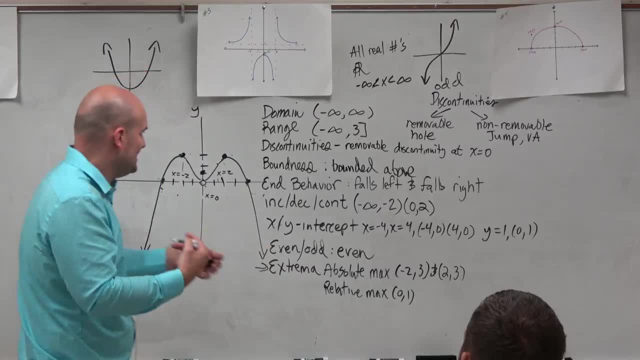 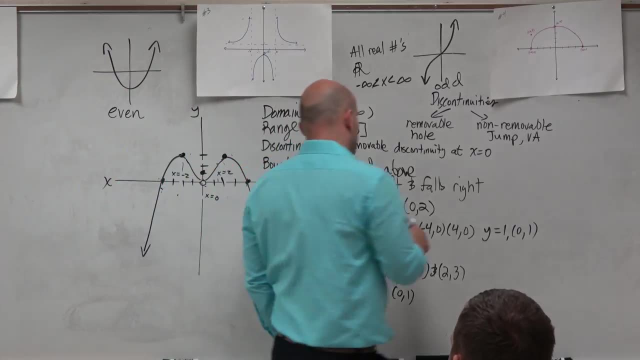 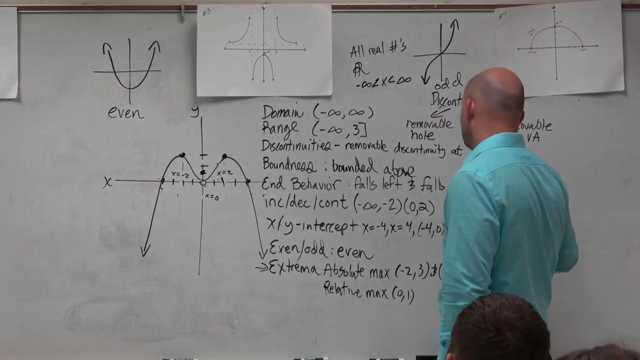 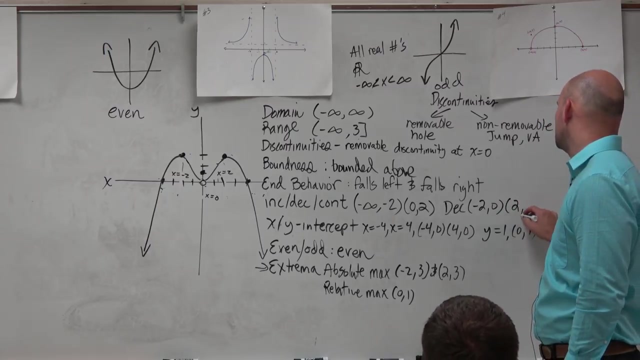 So when you're writing your increasing, decreasing intervals, you're explaining this. You're describing this with x intervals. When is it going up, down or constant? And then it is decreasing on the interval negative 2 to 0, and then on the interval 2 to infinity. 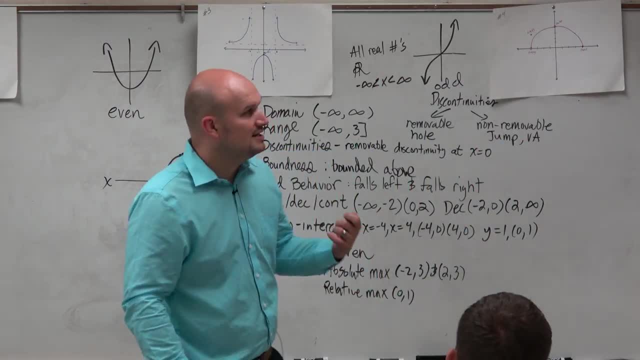 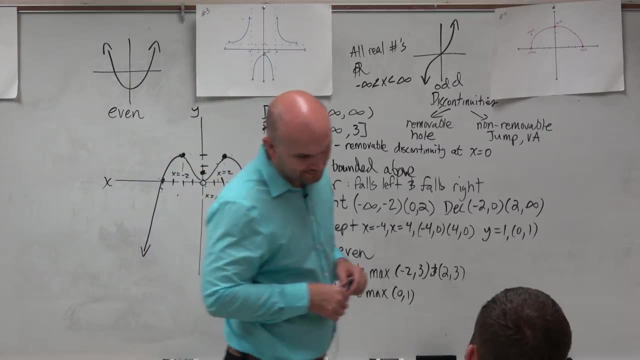 So I spent a whole bunch of time. I didn't really take too much time breaks. Does anybody have any questions or anything that I kind of covered? Yes, So for the graph- you're saying for the maximum and minimum points, do they always have to be in the graph? 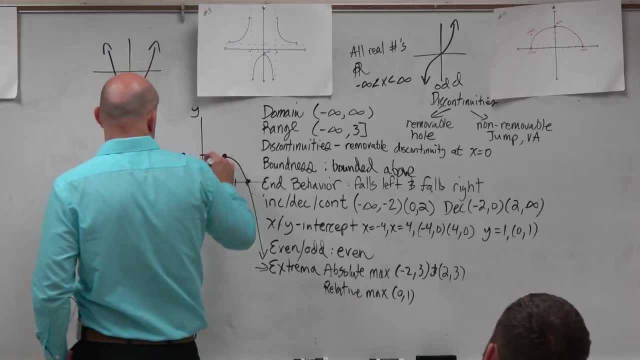 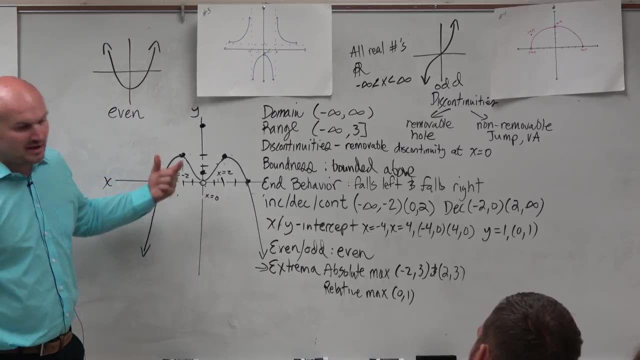 or they can be like that black point. No, yeah, So if I had a point up here, that's my new max. I'm never going to have a minimum, though, at least in this graph, an absolute minimum, because the graph continues indefinitely. 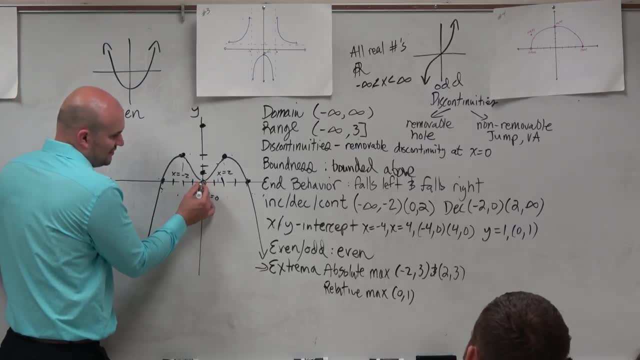 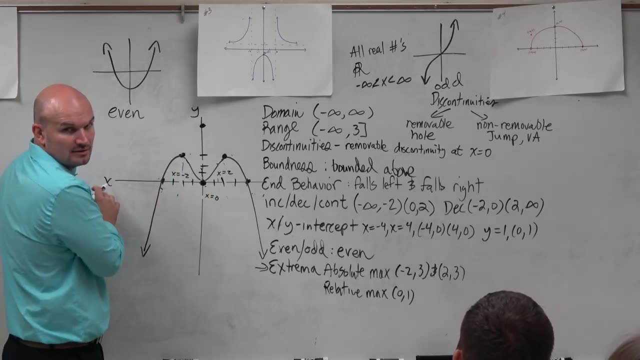 without bounds going down. But, as I mentioned, if this was filled in and that wasn't there, then that would be a relative minimum, because points to the left and to the right are above that. Yeah, so like the two points in the graph. 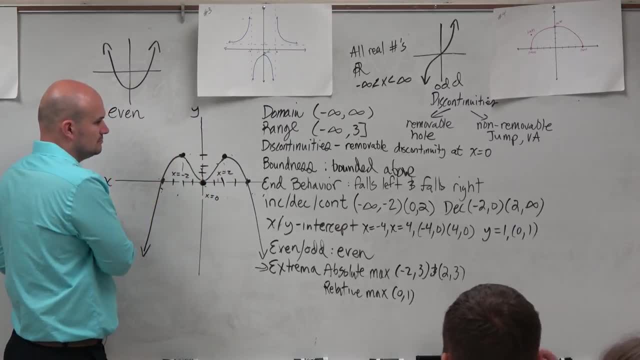 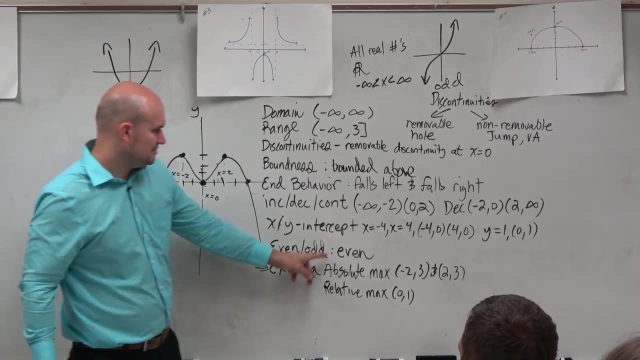 right, Yeah, The two points at the top, how you said, they were both like a max and a min. No, they're just both maxes, They're not both mins. These two points are both maxes. They're absolute max negative 2, 3, and 2, 3.. 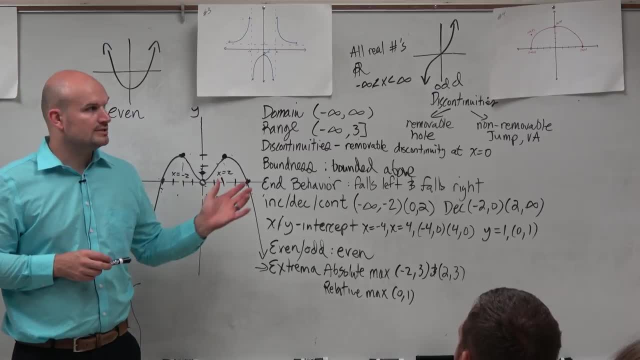 Good, Anybody else? Anything? Sure, Yeah, you can take them. I'm going to leave this on the board too, if you guys need, because we're going to do an activity, All right. All right So.